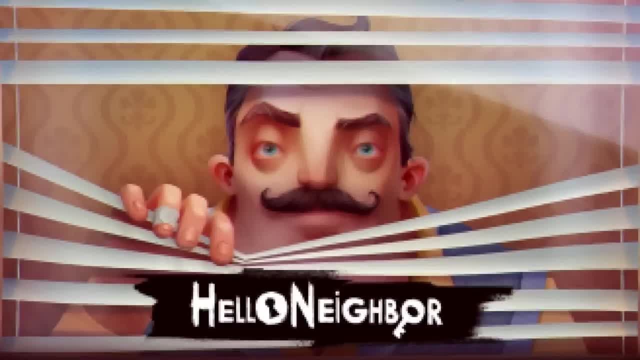 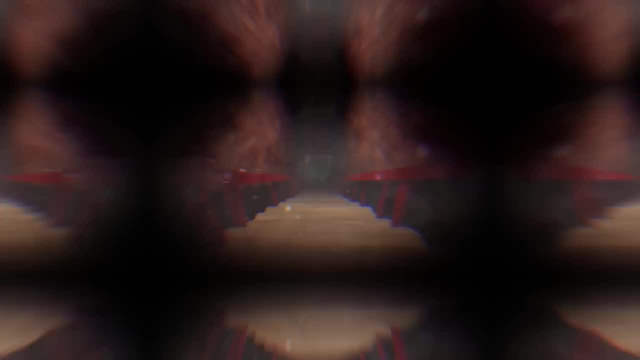 idea what I'm talking about here. let me just bring you up to speed, Hello Neighbor. probably a game that needs no introduction, right? It was an indie horror game that blew up a couple years ago, all about a kid trying to break into their neighbor's house to discover the secrets that 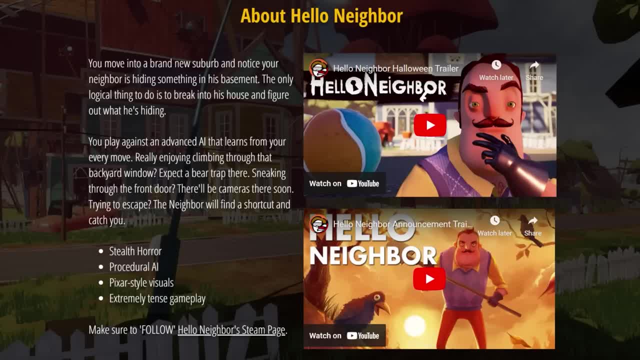 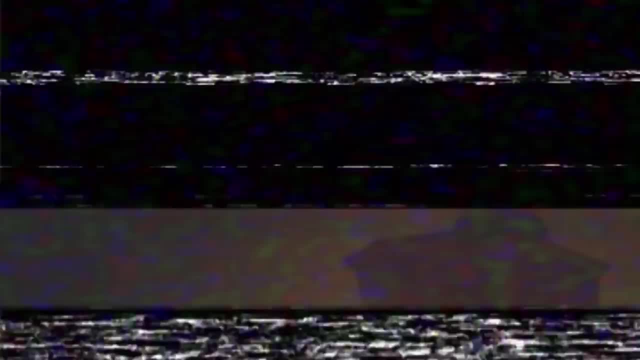 are hidden inside his basement. At the time the devs really hyped up the enemy AI, the neighbor getting to know your routes through his house, getting smarter as you play and getting more and more skillful. It was an idea everyone got really excited about And the story they 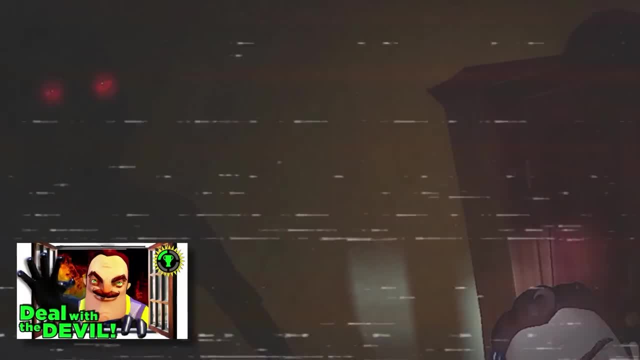 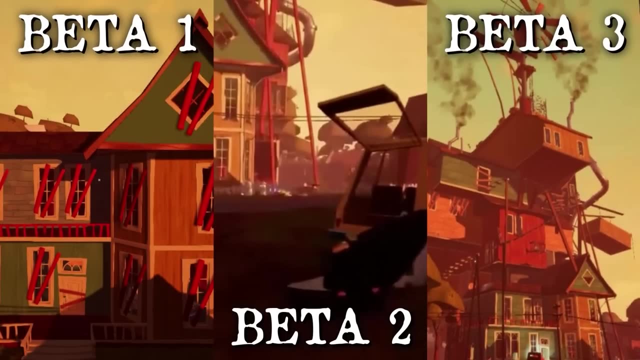 were teasing was also really cool, with images indicating that this mysterious neighbor had sold his soul to the devil. And so they released a pre-alpha, and then an alpha, and then another alpha, and another, and then there were like three or four separate betas, and each time 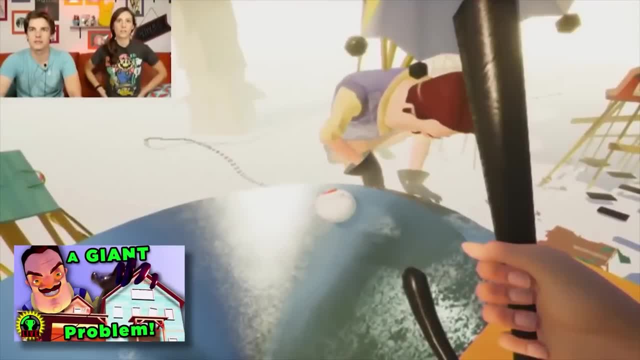 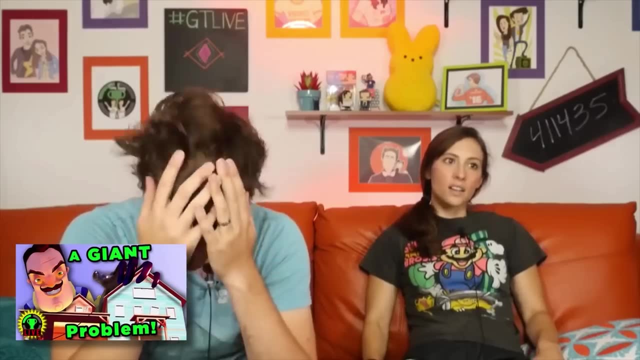 the game was just vastly different and significantly worse. It's not going. The ball is stuck, It's stuck. Why does our copy of the game literally not do anything that it should? Oh my God, Get me out of here. Declare war on me, Get me out. 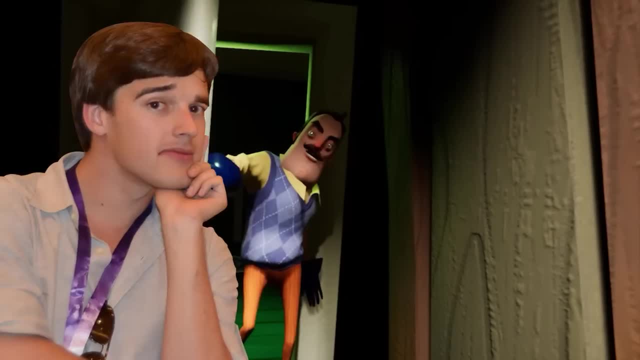 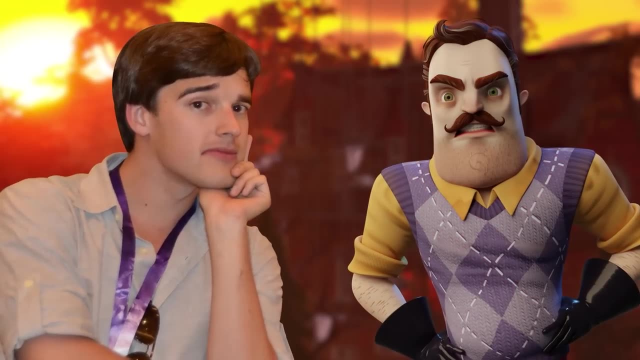 it should be doing until the full game finally released, and it just wasn't good. it was glitchy, the puzzles didn't make sense and the story was incoherent. it was this really big letdown for me for a game that, honestly, i thought had a lot of promise. now i'd done a handful of theories on. 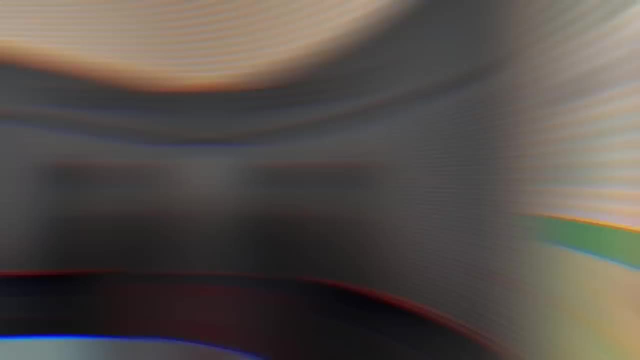 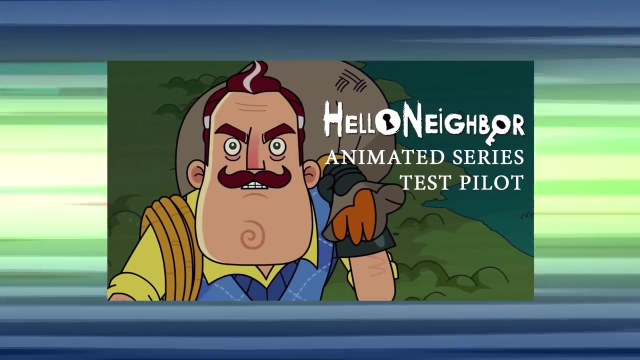 those alpha builds and those really helped the game blow up in its early days. but after being so disappointed over and over again with the various releases, just kind of stopped covering the whole thing. fast forward two years and suddenly there's a new tv pilot for an animated 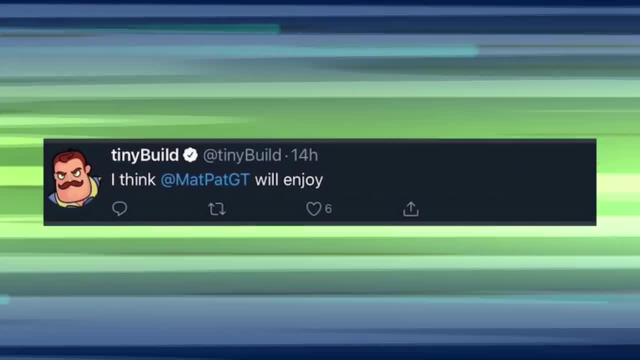 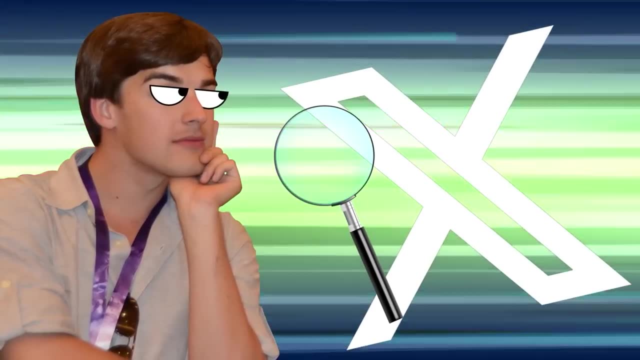 show based on the series and i'm getting tagged by the hello neighbor staff on twitter to not just watch the thing but to analyze it frame by frame, and normally that sort of thing be fine, no big deal. i get asked all the time on twitter to analyze things, but what made this one different? 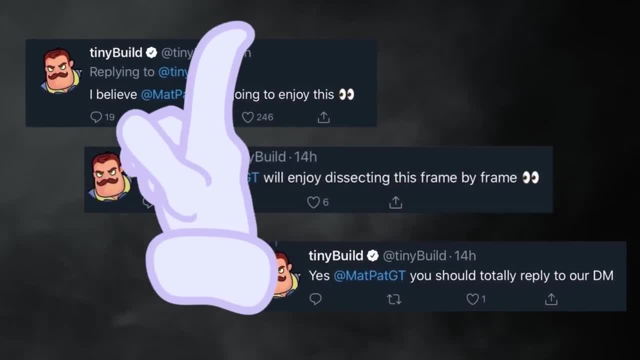 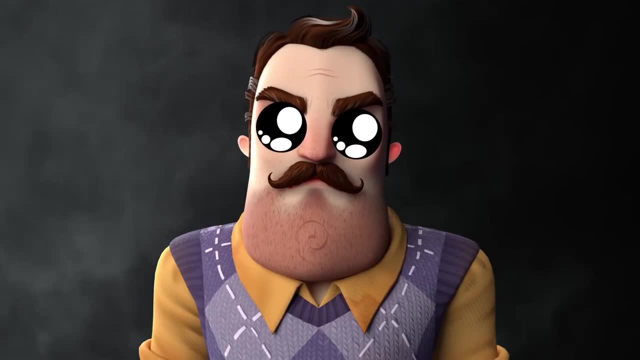 is that they did it over and over and over again, not just once or twice, but three times, back to back to back, basically saying the same thing over and over again. they were practically begging me to do a theory on this thing. the internet would eventually notice this long string of tweets. they 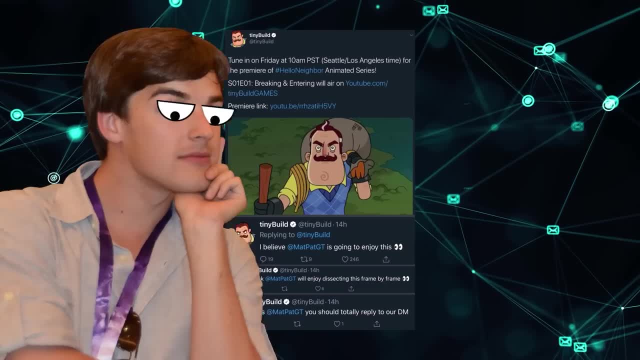 were screen grabbed and then they became immortalized as a meme, as you can see in this video. there's a lot of stuff going on in the internet right now and for me- yeah, i never wound up doing it. i never did watch that tv pilot, nor did i analyze it frame by 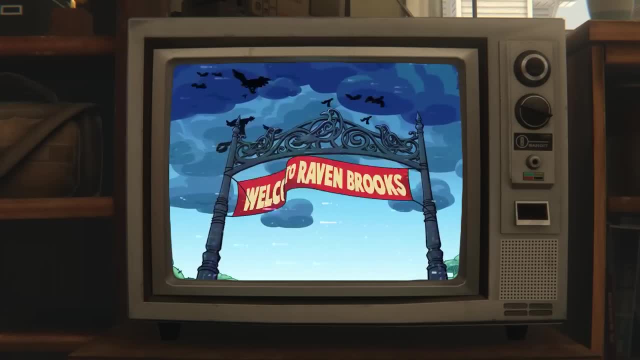 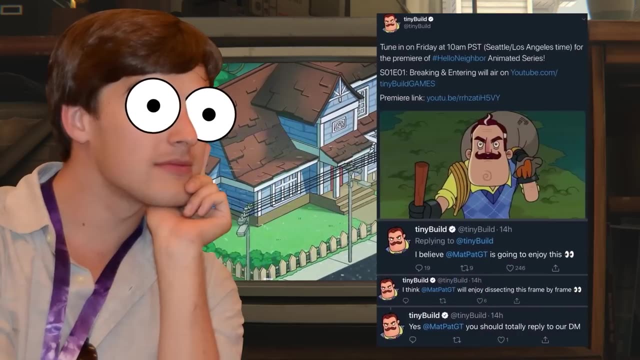 frame, like they were asking me to, until today. that's right. i'm finally going back to analyze this thing frame by frame, four years later, which you know is fitting. i was always late to the meme anyway. but what's our theory looking to do today? what am i trying to prove the deep lore of hello. 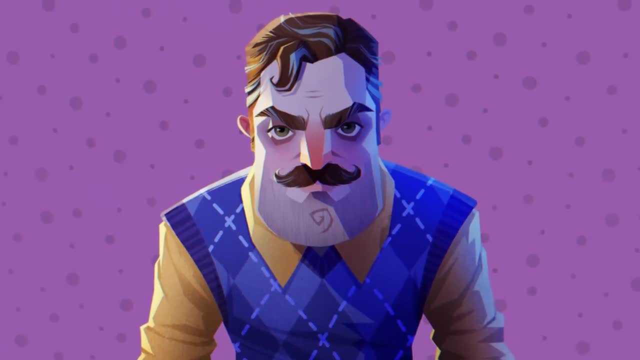 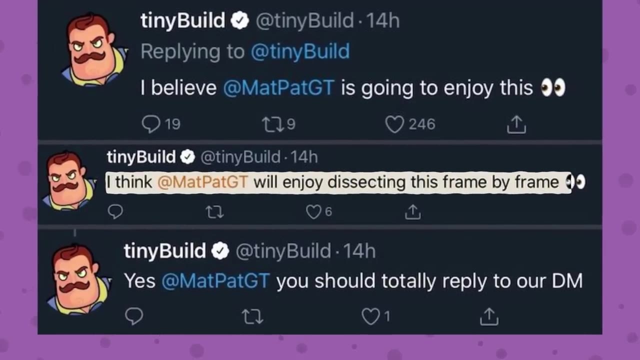 neighbor. yeah, i suppose there's gonna be a little bit of that in here, but the real question that i wanna answer today is whether or not i enjoyed it was tiny, build right. would i have actually enjoyed analyzing their tv pilot frame by frame? in total, there are 8748 frames of this thing, so, uh, we better. 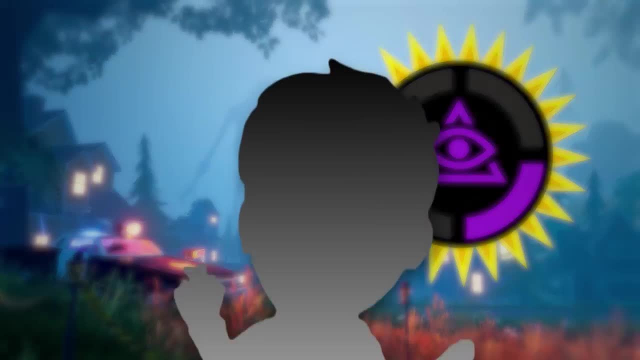 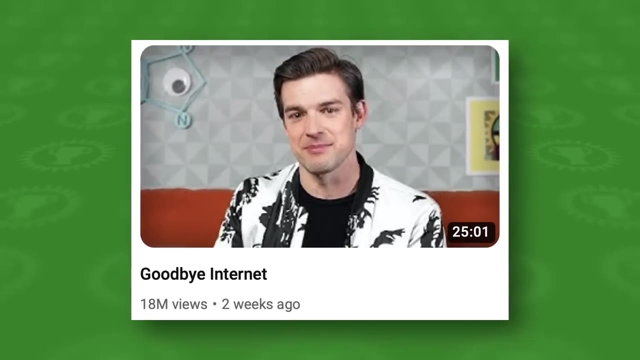 get to cracking. but before we get all conspiratorial with the pilot, i first got to tell you about something else conspiratorial. some of you have already been putting the pieces together over on twitter, but now i can confirm, as part of my retirement from hosting the channels, i finally 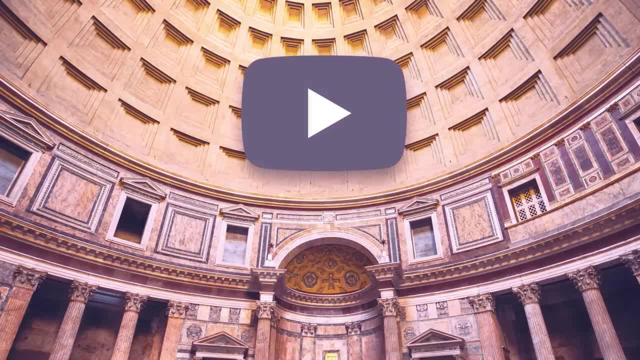 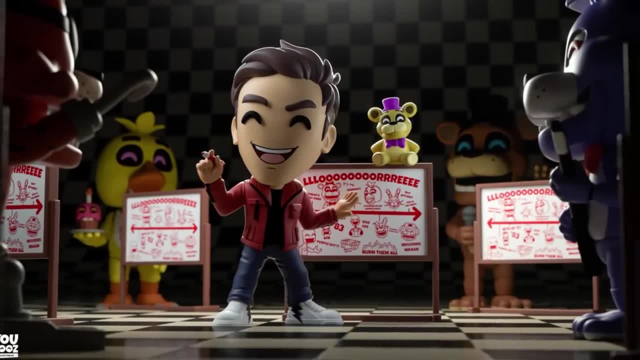 have my very own youtube's figure. that's right, my friends. i'm finally immortalized amongst the pantheon of youtuber collectible figures. look ma, i made it. i worked together with the youtube's team to really personalize it into something that was million dollars worth of money, and i couldn't do it. 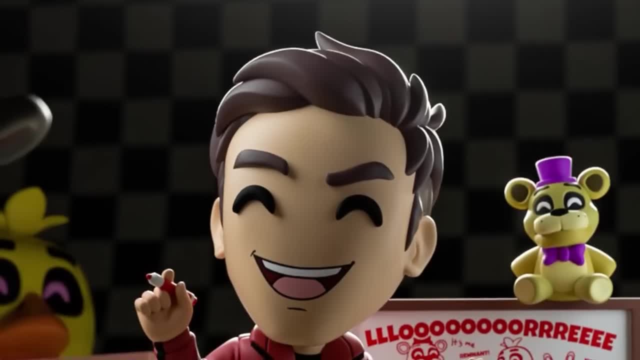 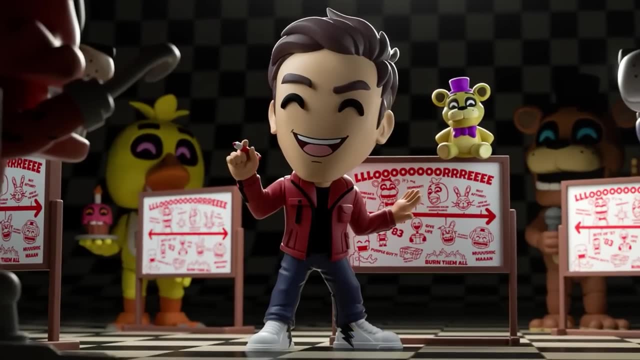 Every element of this figure: iconic red jacket, the hair swoosh, my favorite pair of shoes, even the smile that I put on when I'm Dying inside trying to solve the FNAF timeline. but you're not just getting me my friends with this, you twos. 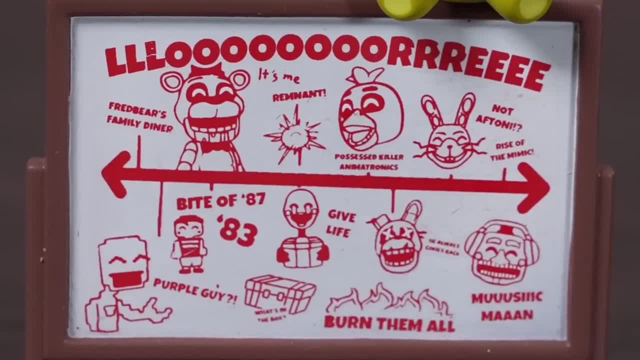 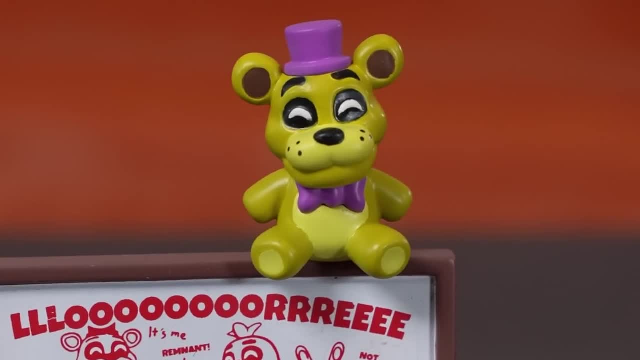 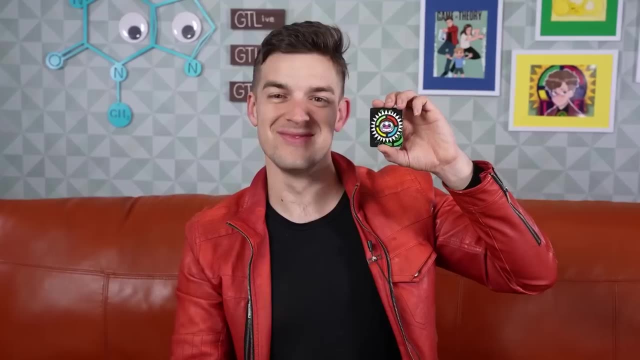 You're also getting my very own conspiracy board. This thing is chock-full of little Easter eggs for you to discover. plus, I had to be joined by my original best boy, the absolutely iconic psychic friend Fredbear. here He's, there He's everywhere. Who you gonna call psychic friend Fredbear? That's not all. for all your pin collectors out there, 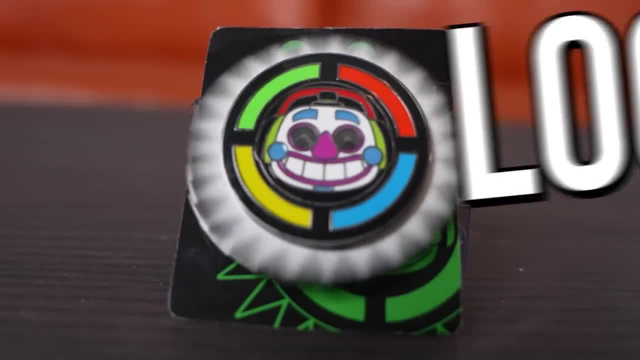 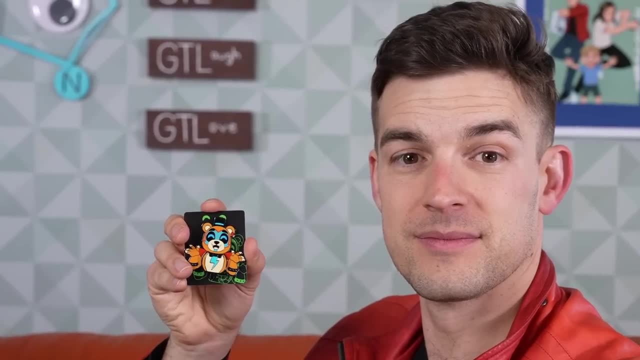 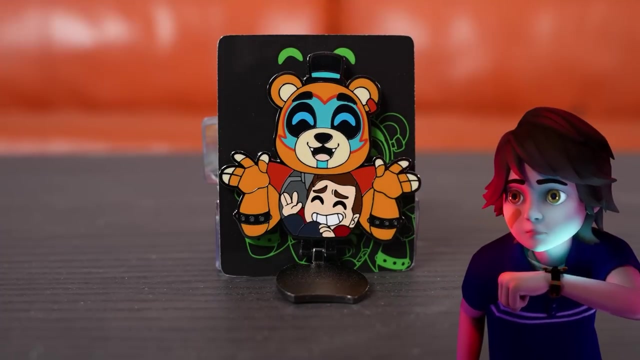 There's also these incredible spinning pins. now You can have me shouting to music man Anytime and anywhere you go. my personal favorite, though, has got to be this one of me becoming a meat pretzel inside of glam rock. Freddy's Stomach hatch- look it, even opens and closes- must be like some sort of robot kid. now, if you don't know how you twos works, 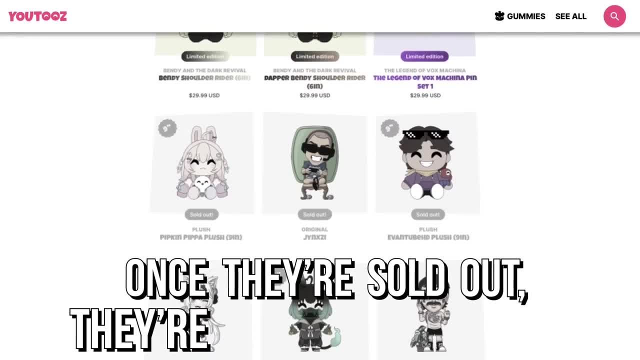 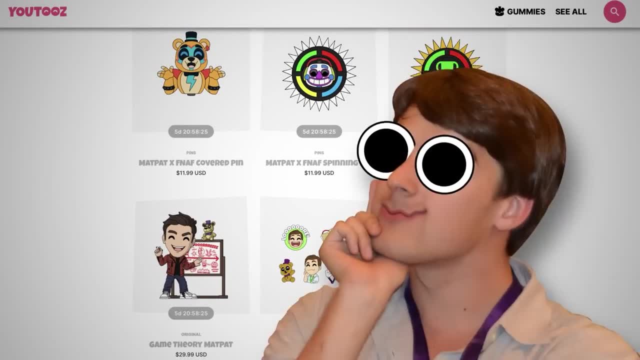 These are all limited edition items, in other words, once they're sold out, They're never coming back. There's a countdown clock and everything, which is why it felt fitting for them to be one of my final merch items. feels poetic in a Way. So grab yourself a little piece of history before they and I are gone forever. 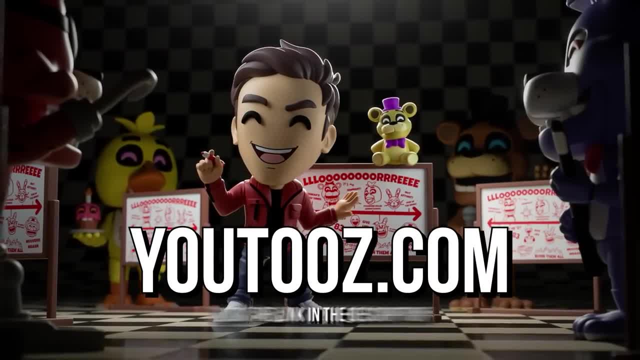 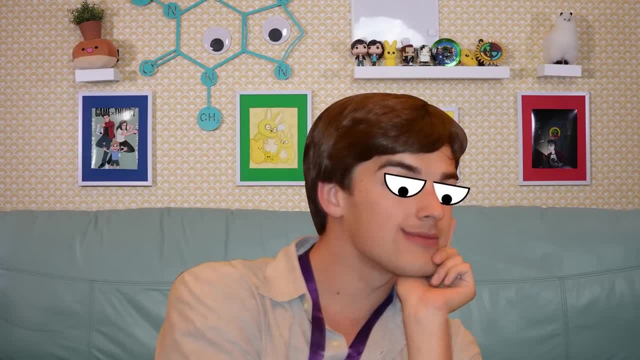 They're all available right now at you twos Dot-com. hurry down to the description and click the link to get your little matpat. while you can now, then I'm gonna take my seat Right here on the couch. We're finally gonna take a look at the YouTube pilot episode for a game about the scariest thing of all. 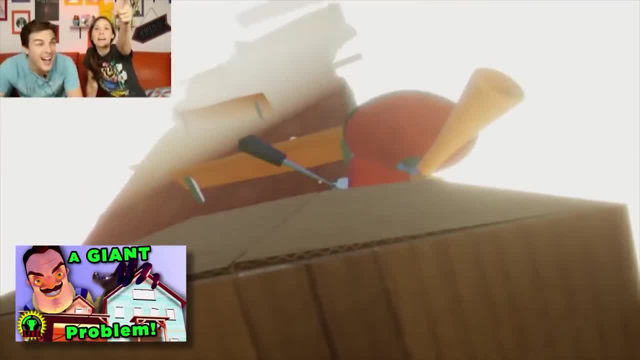 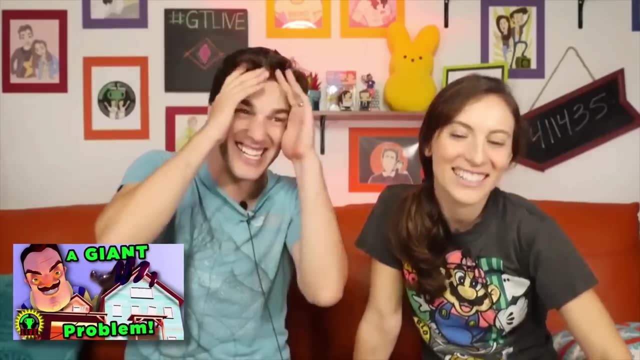 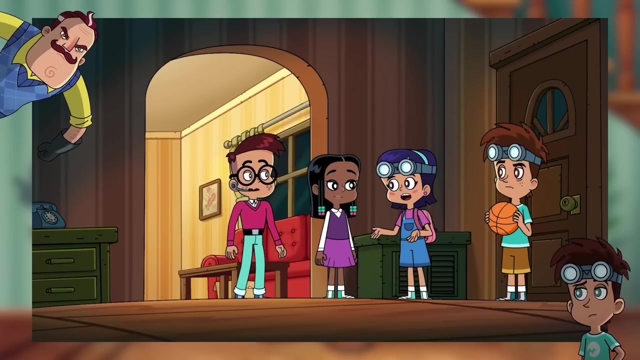 stacking boxes, The ultimate box stacking. you've got to stack the boxes all the way up there. final boss isn't a giant neighbor. the final boss is The pilots. only five minutes long, But it gives us a pretty solid foundation of what the plot of the show would be. follows a group of kids who are all suspicious. 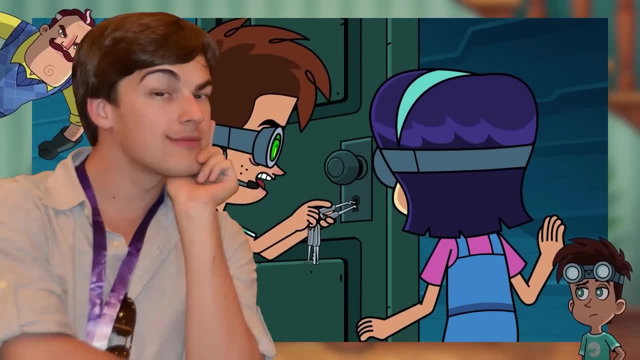 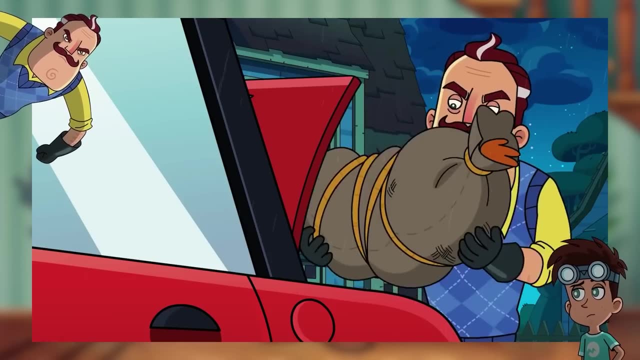 Of the neighbor, so they decide to investigate his home to see what they can find. of course, It doesn't quite go according to plan. the neighbor tries to catch him, but using his own house against him, They're able to escape. the kids watch as he puts a body into his trunk and drives off curious. 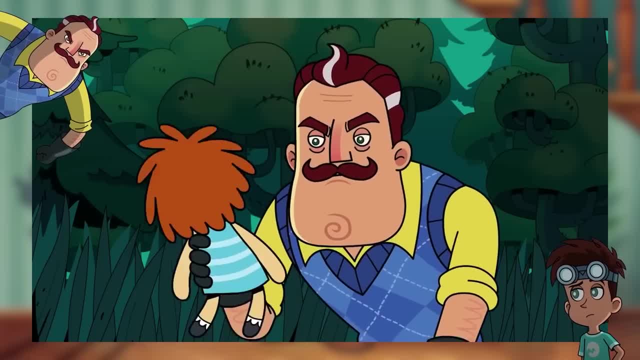 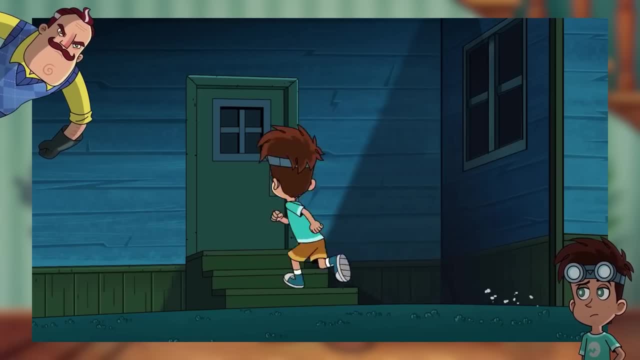 The kids follow him and discover that it wasn't a body after all, but rather a doll that he then promptly Buries. the neighbor yells at the sky for a bit, realizes that the kids are watching him and then chases him away. They once again escape, racing home before the neighbor. does they watch? 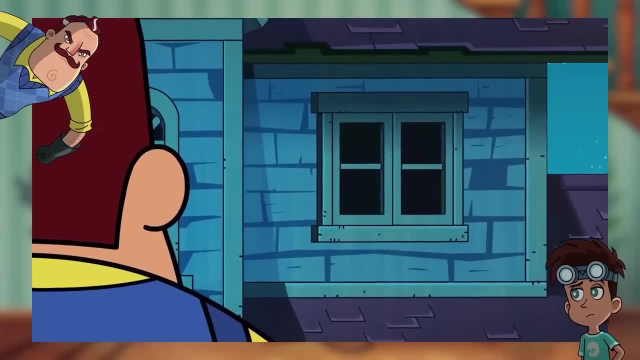 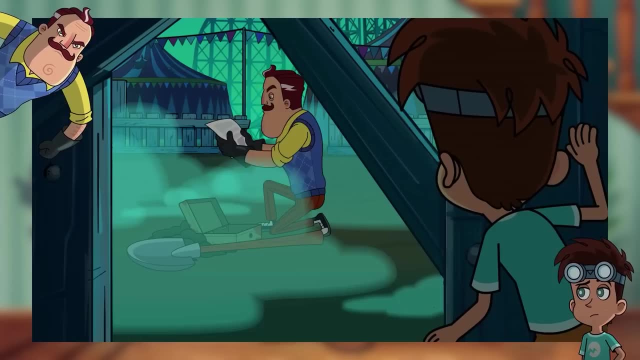 Him from the window until, of course, the neighbor turns and stares back. cut to black. It's short, It's sweet. it captures a lot of the feeling of the original game. It's got secret passages, a mysterious but angry neighbor and, of course, a mystery about what the heck is going on with this guy. 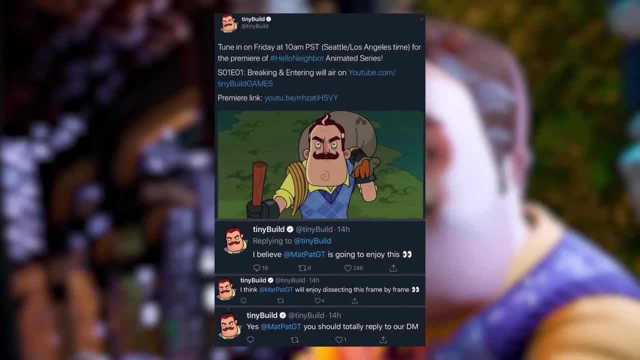 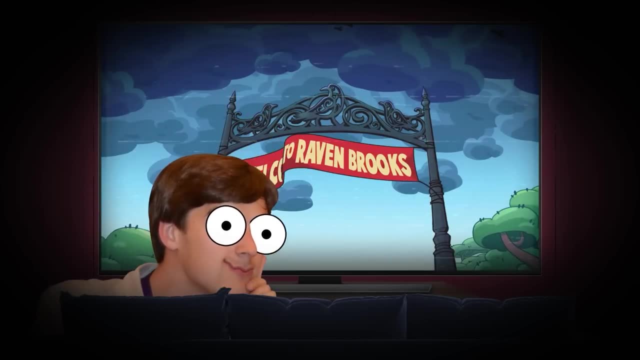 So if we want to figure that out, we got to do what the meme suggests and go through it frame by frame. Here we go, Okay, so right here at the start, frame five, Telling you we are doing this. it's gonna be a long video here. 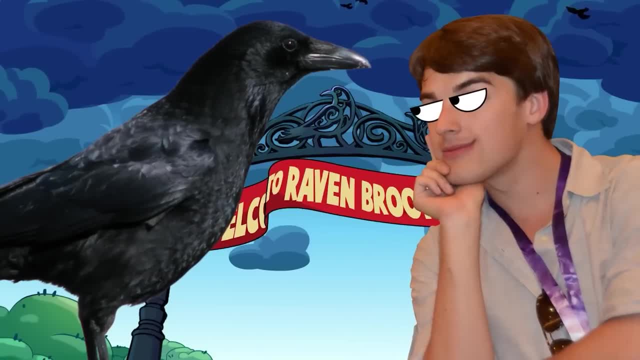 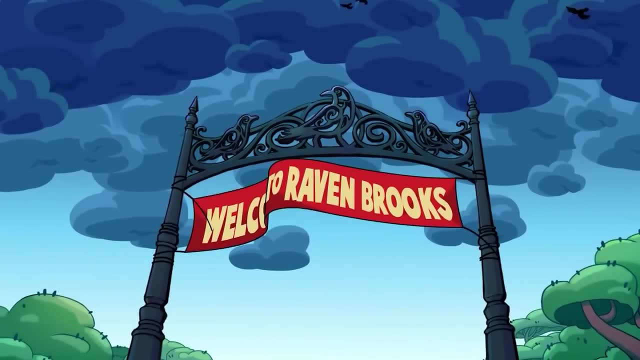 We see the return of hello neighbors favorite creature, the crow. I never really spoke about crows in my initial theories, But they are Everywhere in this franchise, from the concept art to pretty much every installment of the game, and now they're here too. Usually, these guys are just set dressing. 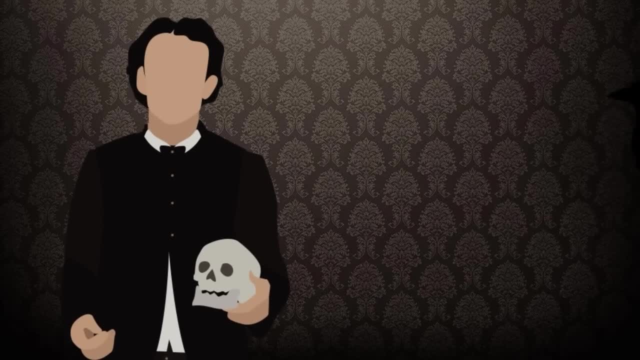 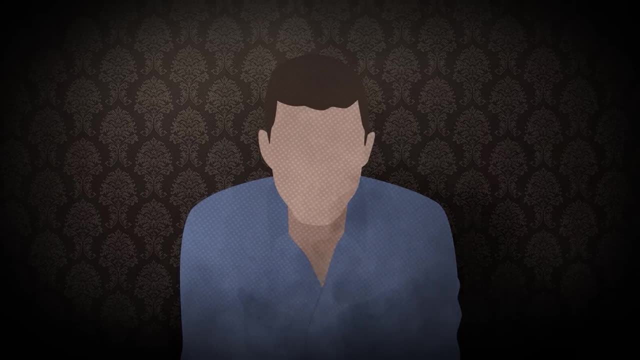 But I would suspect that the connection here is actually deeper than that. Edgar Allan Poe famously used a raven in his poem the Raven to be a stand-in for bad omens, a reminder of all the bad things that happened in the main characters life in this. 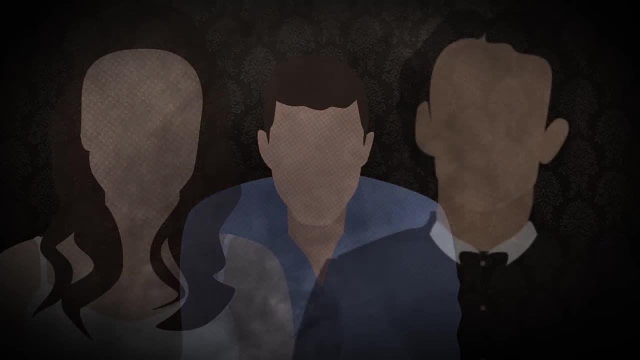 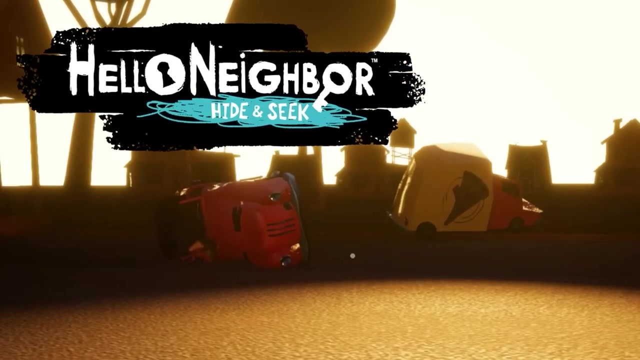 Case the death of Lenore, a stand-in for Poe's dead wife Virginia. and all of this is very fitting when you consider that mr Peterson also loses his wife in a car accident during the events of hello neighbor hide-and-seek, which takes place before. 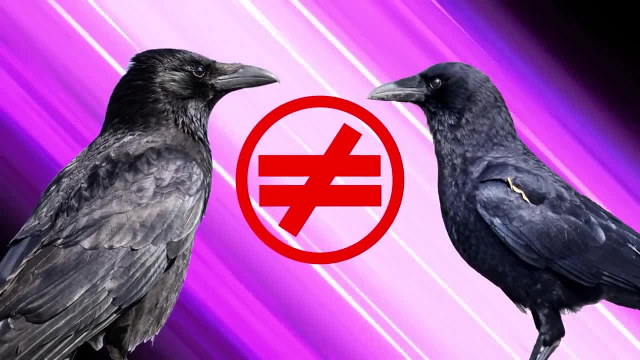 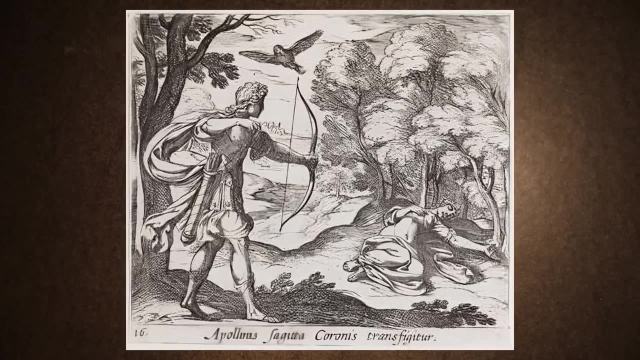 Act one of the first game. also, I know Ravens and crows are technically different, But in a lot of old mythology where these sorts of ideas originate the two were often used Interchangeably. Greek myth, for example, claims that it's crows that are bad omens, giving the god Apollo bad news. well, in Norse and Celtic mythology, 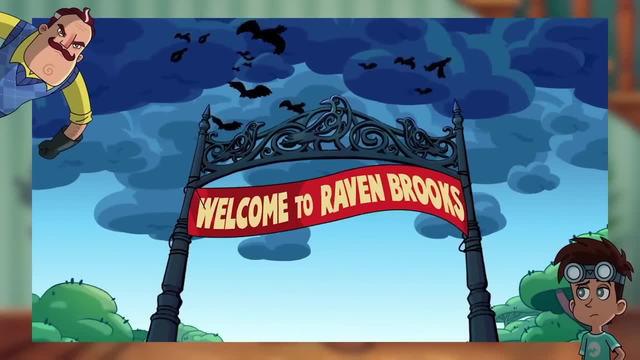 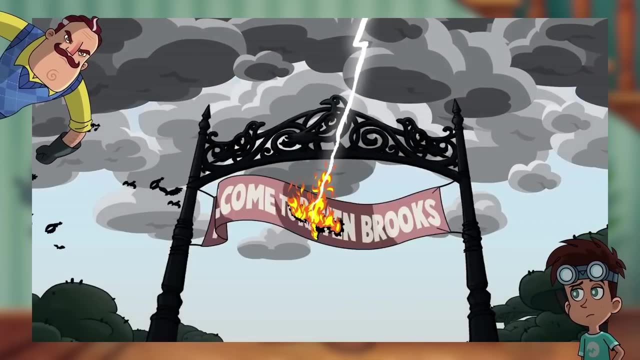 It's a raven. That's a sign of war and death. so, starting off the opening shot with crows and ominous dark clouds, not the best sign for whatever's gonna Happen? and if the crows weren't enough, the lightning that strikes the banner at frame 39 is just icing on the cake. very spooky indeed. 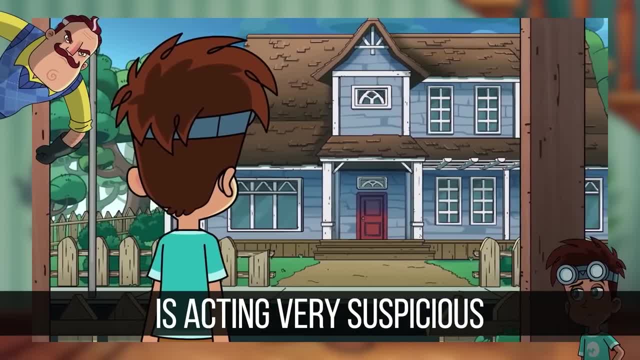 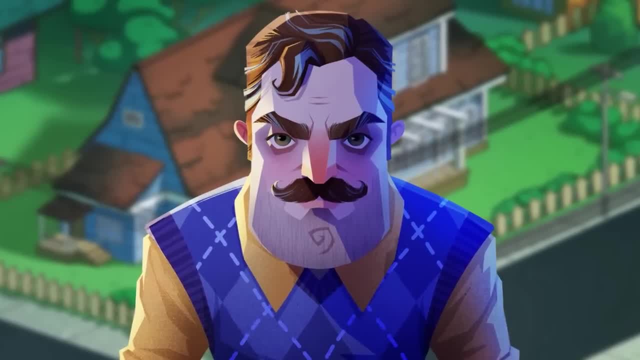 My name is Nicky raw. my neighbor, mr Peterson, is acting very suspicious after his children, Aaron and Maya, gone missing. all right, There's lots to unpack with this one. first, the neighbor has a name. I've been referring to him as the neighbor for all these years. 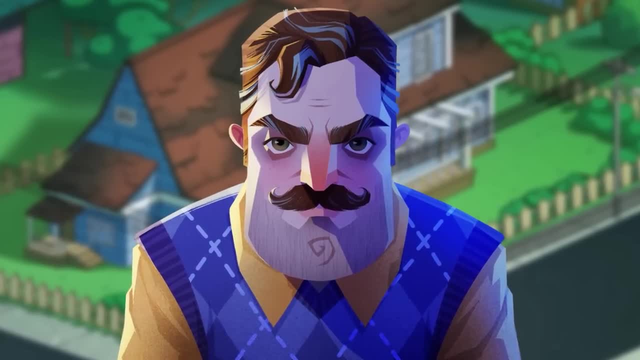 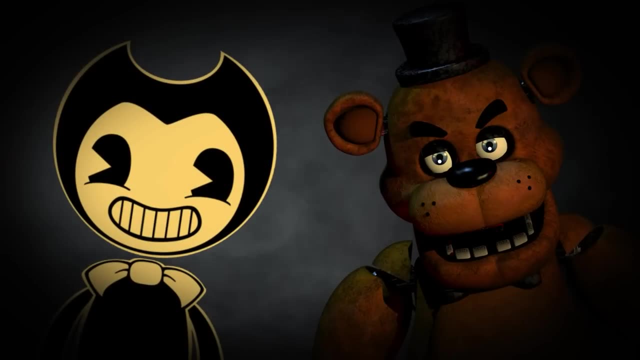 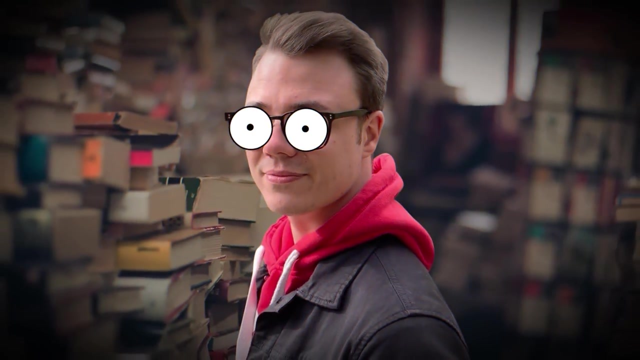 But apparently he's had a name the entire time. according to the hello neighbor books, his full name is Theodore Masters Peterson, and you heard me right the books. like every other indie franchise these days, hello neighbor broke off into its own series of not Just one, not just two, but seven books. fortunately for me. your new game theory. 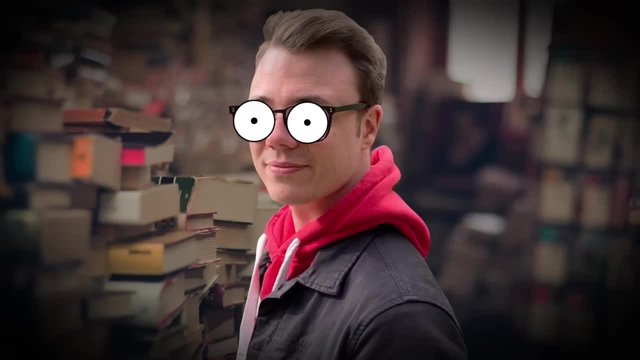 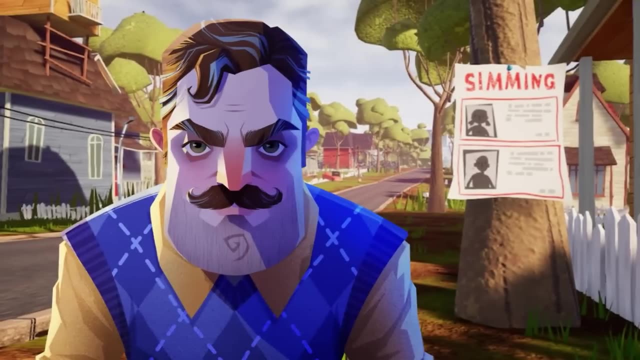 Host Tom was insane enough to go and read the entire book series himself. Thanks for saving me on that one there, Tom. if you think I'm insane, just wait till you hear what's in these books. But it is pretty weird that such an important piece of information like your main characters name just isn't in the games agreed. 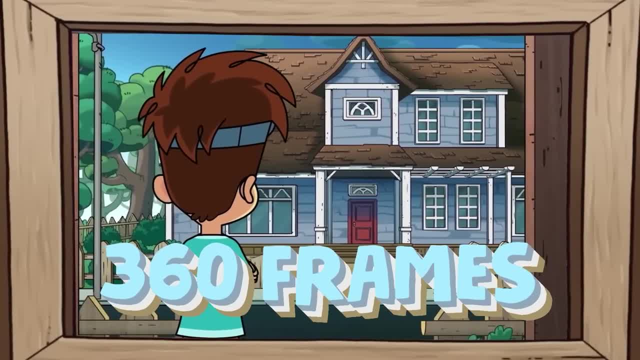 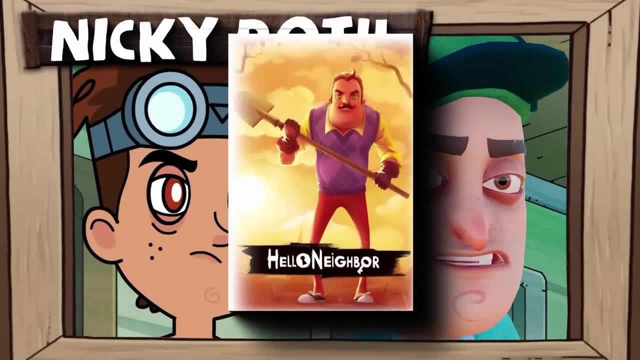 Okay, now here We are. we're 360 frames in and we're already being shown when, in the hello neighbor timeline, the show takes place. you might not recognize him, But this guy here, Nicky Roth, He's our protagonist from the first game. He's missing the baseball cap in the large jaw. 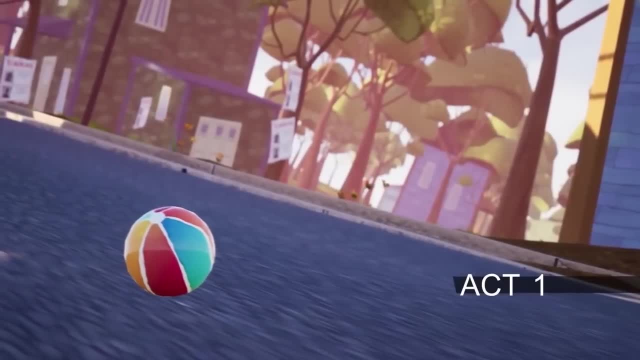 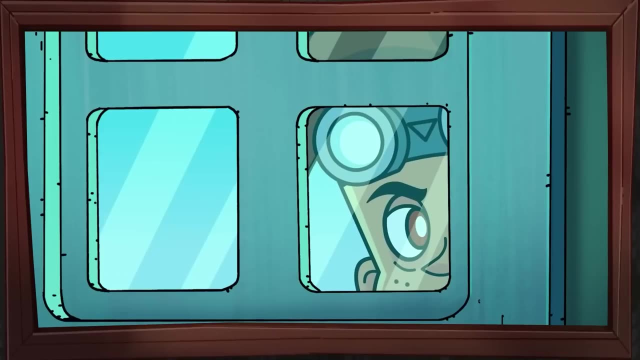 But he still does have that iconic chin swirl, an act 1 of hello neighbor Nicky's kidnapped and locked in the basement, only Escaping years later and not returning to town until he's an adult. if he's out here spying on mr Peterson as a kid, that means that this show has to happen before the events of act 1 in the first game. 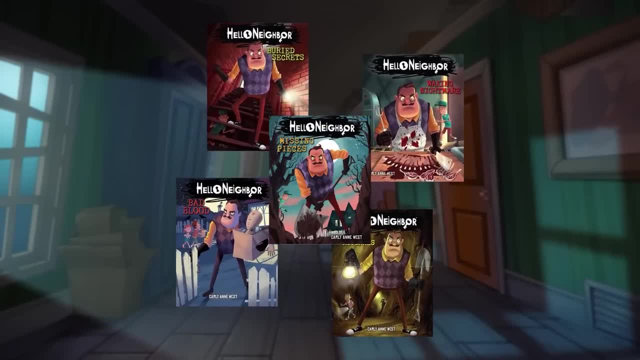 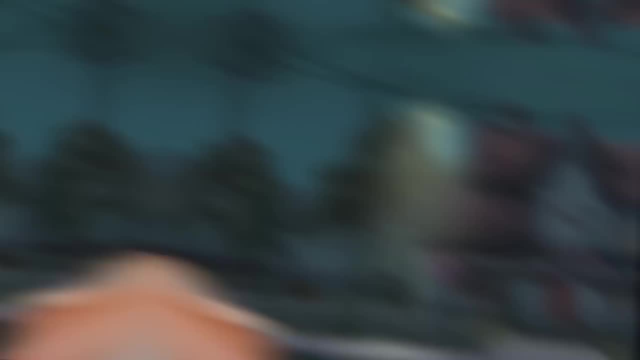 Which you know is great because, again, outside of the books, We get very little information about this part of the game, or really any part of the game, for that matter. So who knows, maybe this will be able to answer some of our burning questions about this franchise. one last thing, by the way. 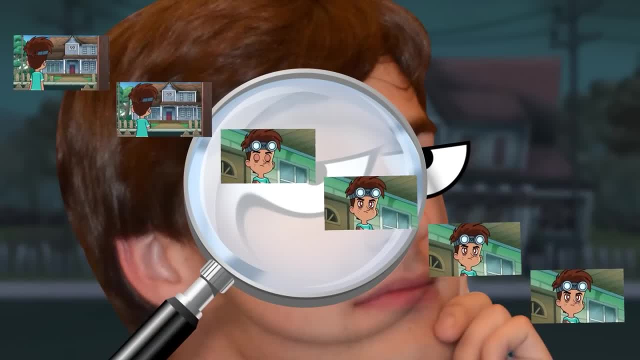 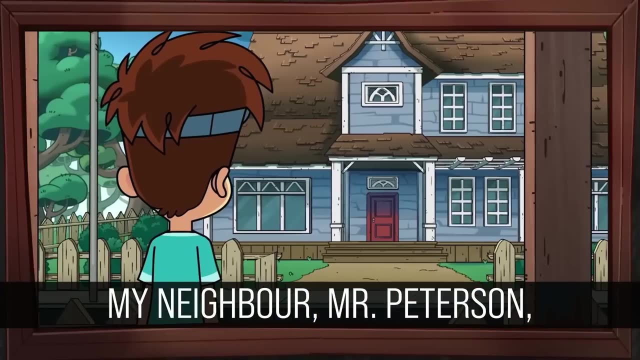 It's less of a lore thing and more just because I'm analyzing this frame by frame And reacting to it the way that I normally would got to point out that my script here is really not happy with the grammar Of that opening line. my neighbor, mr Peterson, is acting very suspicious after his children, Aaron and Maya, gone missing. 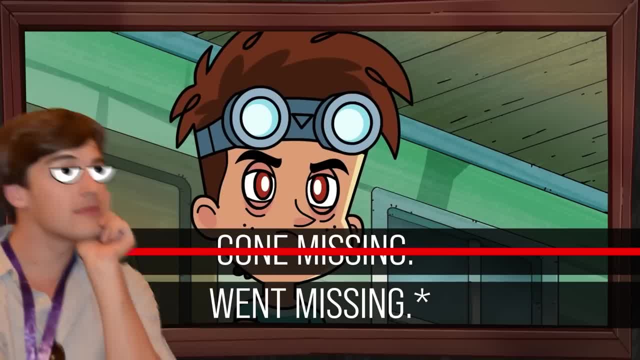 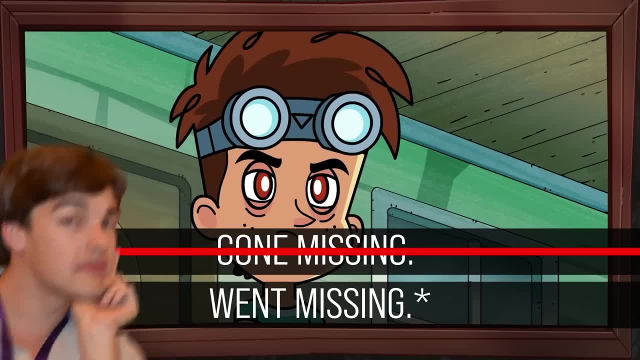 It should be went missing, not gone missing feels like maybe the opening was originally longer And then they had to cut it down, which led to weird grammar and hacky sentences. anyway, It's a minor thing. It did feel weird to me as just an opening line for this franchise, but hey, let's get back to the lore. 430 pm. 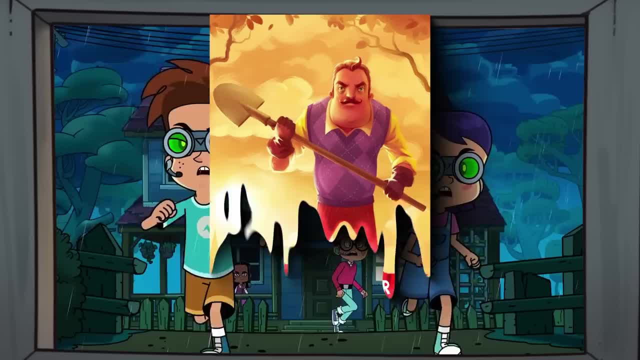 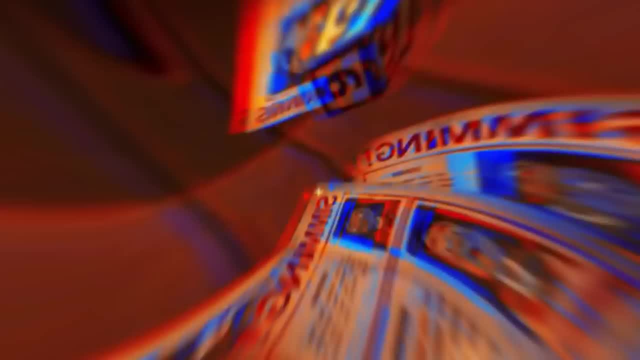 Hall of Records interesting, so the series seems to not take Place in the same world as the games. the original alphas of hello neighbor used Russian for any text assets, and later releases used a made-up Language that jumbled up and swapped around letters. but this it's just an English that, or they just changed their minds. 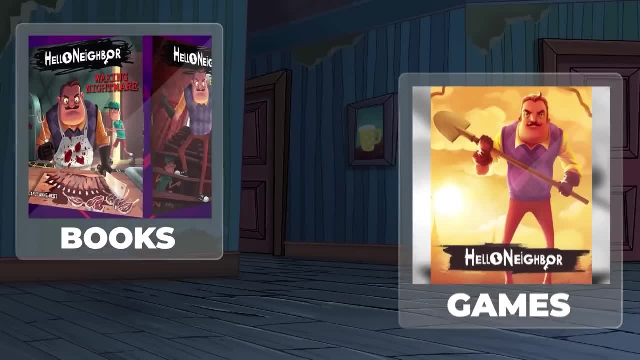 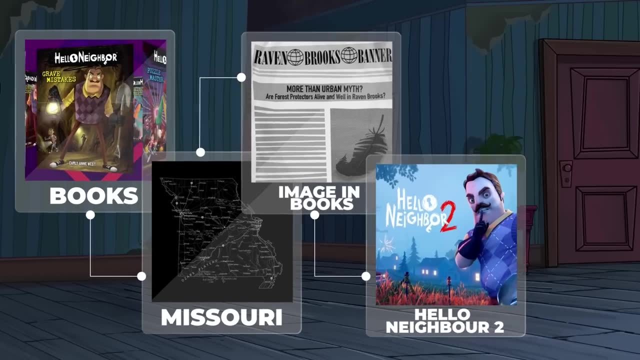 The books are designed to be direct tie-ins to the games And they do take place in Missouri, with all images inside the books, using regular English for all the signs and newspapers. But then hello neighbor 2 came out after the books and yet uses the same mixed-up language as before anyway. 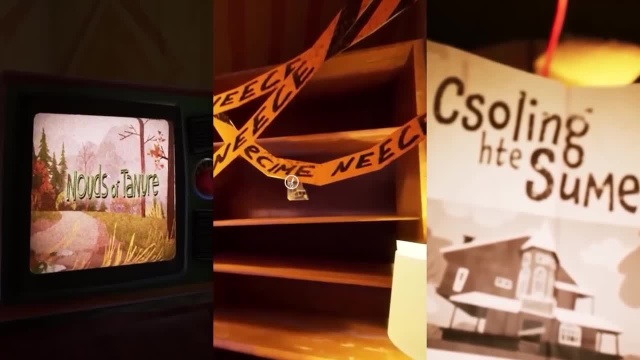 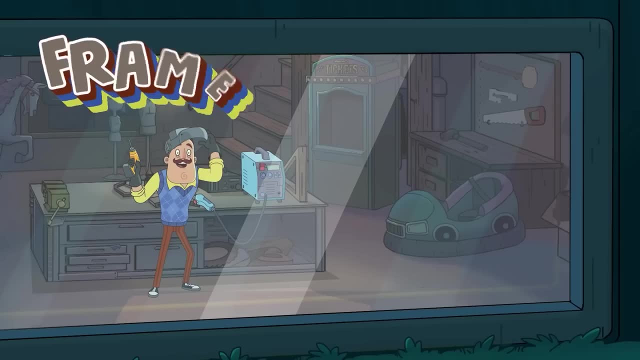 It is very inconsistent how they use text in this franchise. So just make up your mind, guys. you see this. This is why we can't have nice things. 3: 47 am Soldering in basement frame 890. this one stood out to me as odd for the first time. 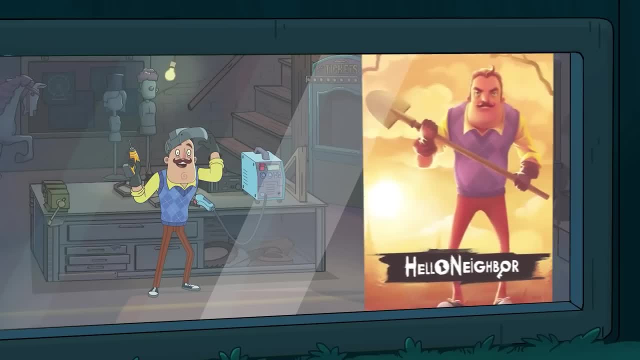 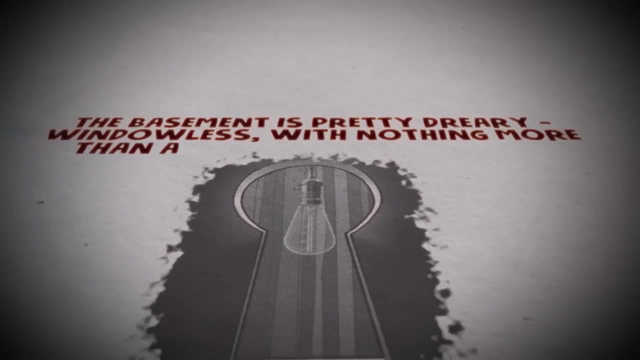 We can actually see into the basement without going inside the basement. in both the games and the books are specifically called out as having No windows. quote from the book bad blood. the basement is pretty dreary, Windowless, with nothing more than a hanging bulb here and there, and in the games 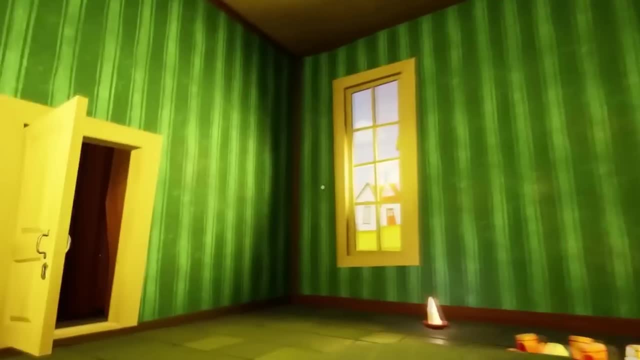 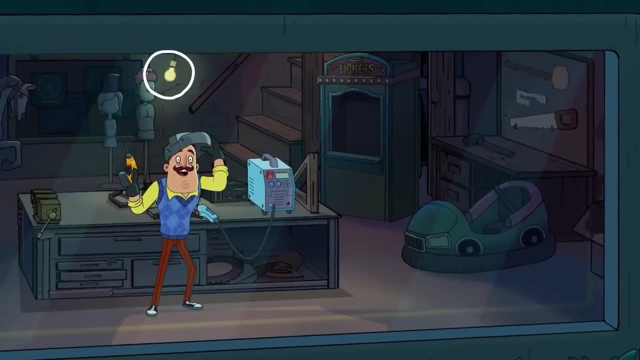 We literally see fake windows with drawings of the outside world pressed up against the stone, something that the books tell us were made by Mr Peterson's son, Aaron. we can see the hanging light bulb that was mentioned, But the fact that Nikki can see inside the basement does ruin a lot of the mystique that both the games and books tried to. 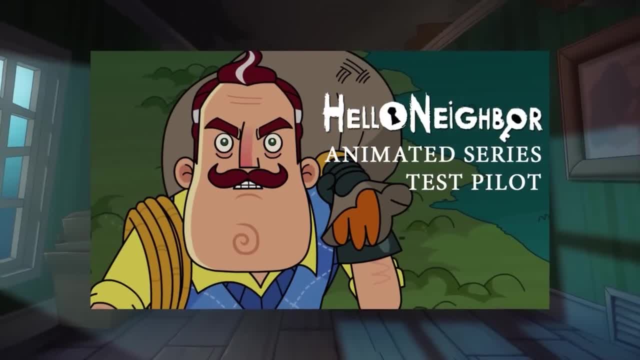 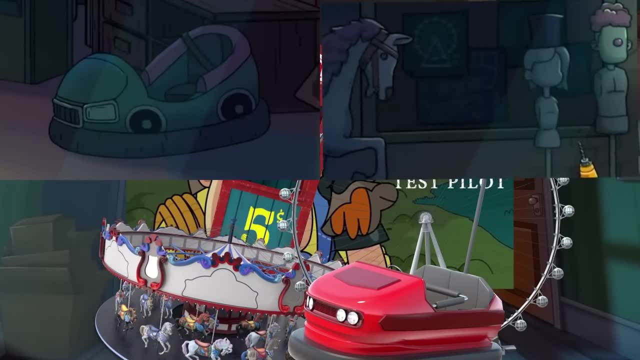 Build up about this mysterious room in the house. however well, It's certainly weird for the story. it does help us theorists because it's full of interesting details, namely that it's full of amusement park attractions. We've got a bumper car, a carousel horse, a ticket booth and a bunch of schematics on the wall for things like a ferris wheel. 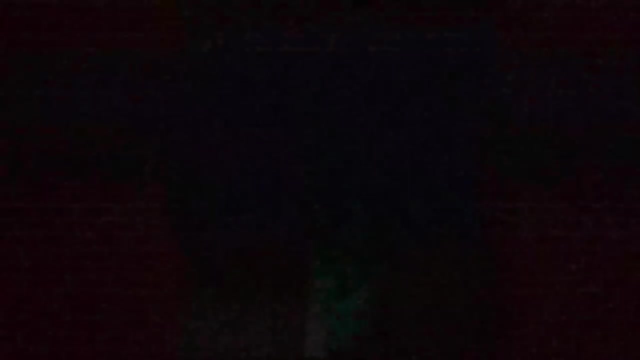 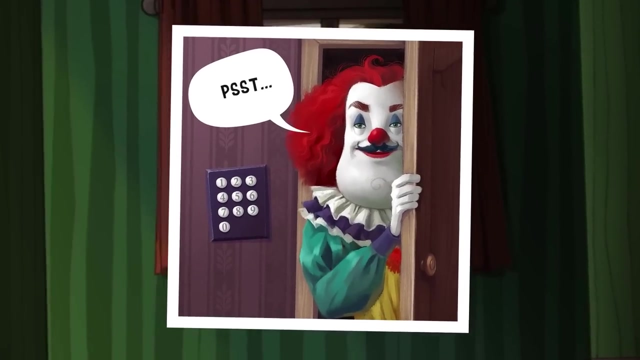 This ties in with what we saw during the very first teasers for this game, where we see mr Peterson wearing a clown outfit back in the day, when I was actively covering the series. I was always confused about that detail, because it didn't tie into anything else. 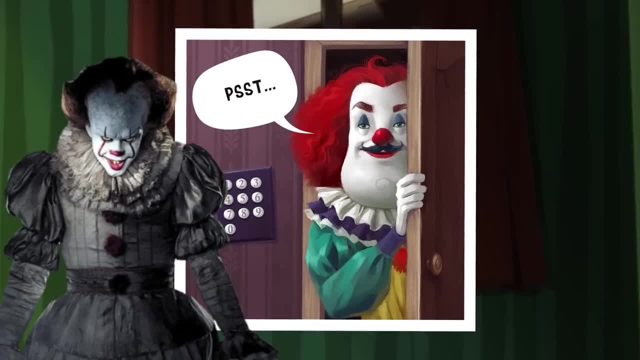 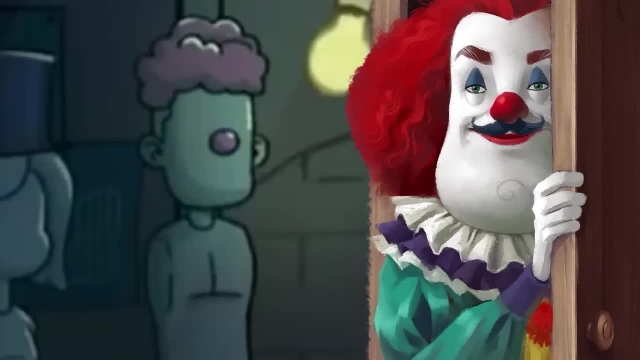 That we were being shown, other than maybe a possible connection to Pennywise, the evil clown from it. But now it starts to make sense when you look behind him and see that on a mannequin is a red nose and red wig- The outfit for a clown. he is actually a part of this circus themed amusement park. 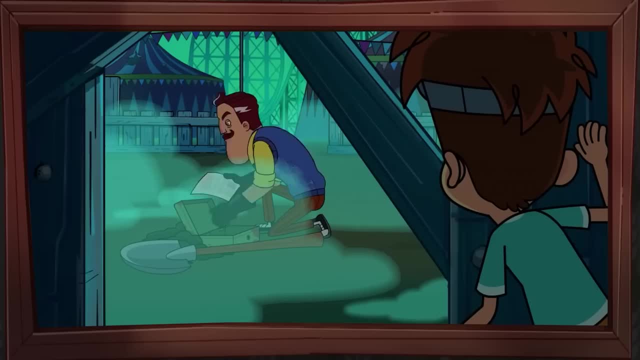 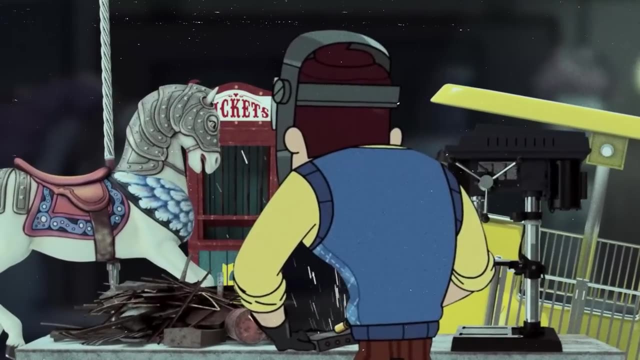 My gut would be the Golden Apple amusement park that we saw just a few frames earlier. and lo and behold, my gut was right, Because the books tell us exactly this: Tom, take it away. So yeah, mr Peterson is the head engineer in charge of designing all the rides for the park. this scene, with the carousel, ticket booth and ferris wheel does. 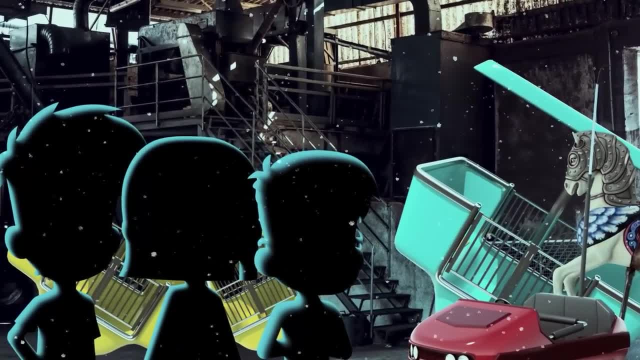 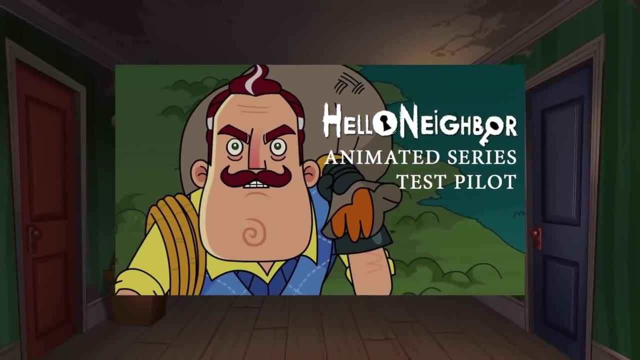 Actually happen in the books, But it's during a class trip to the Golden Apple factory where they're being shown all the designs and plans for the park. that might not seem like an important distinction to make, but What it shows me is that this series is handling things differently than the books, while the books are designed to be a direct link. 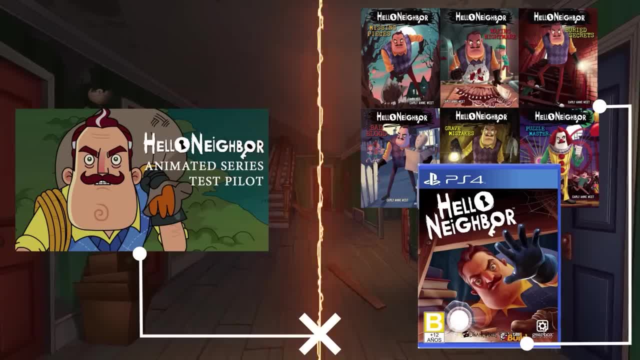 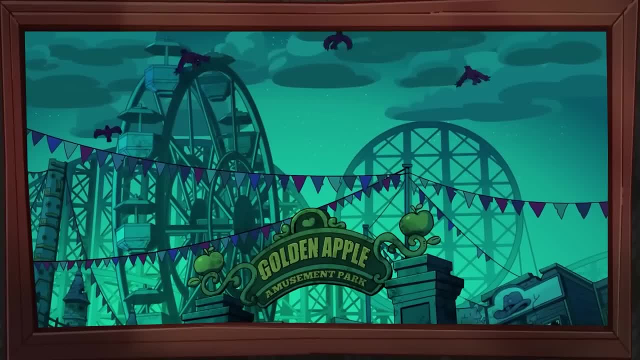 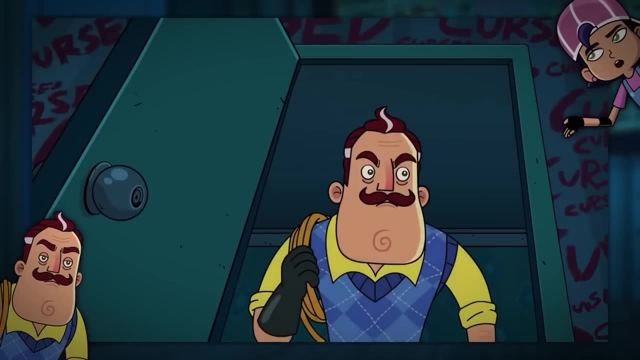 To the stories of the games. this series isn't a direct continuation or standard retelling. instead, It seems to be a reimagining, taking inspiration from the books and combining certain elements for clearer storytelling, But altering it just enough that we get new law. We've skipped ahead a bit, but this is where things get really interesting. 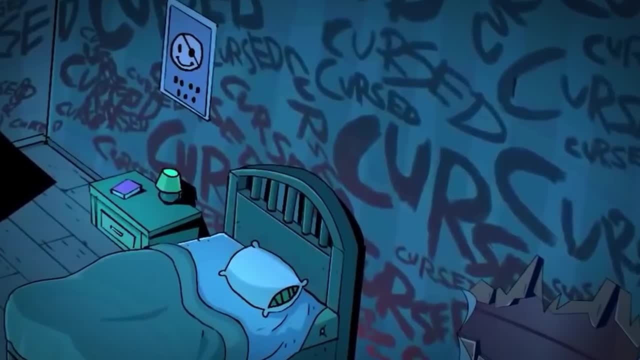 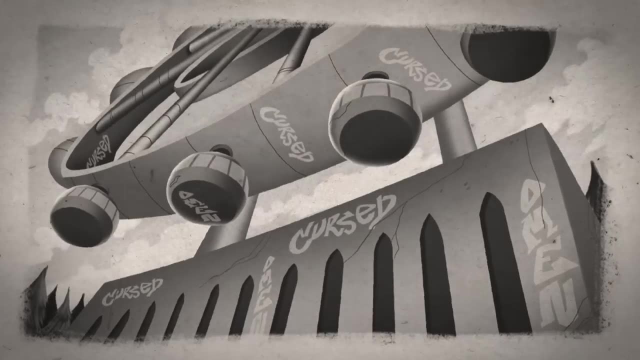 As you can see across the room, We see the phrase cursed written all over the walls. cursed, along with the word omen, are regularly seen throughout the books Graffitied over both the Golden Apple amusement park rides before it opens and on the Petersons house years later. 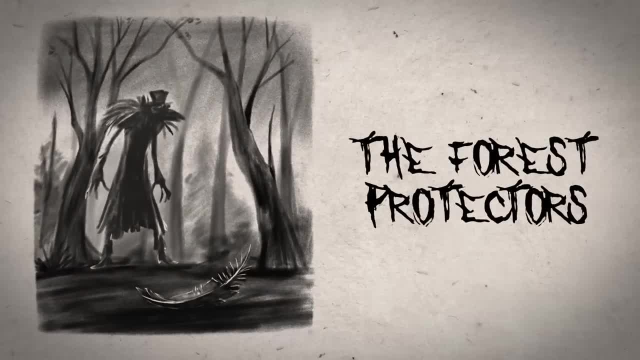 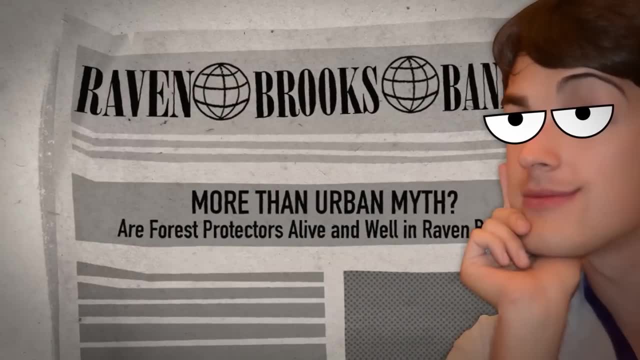 Typically, these phrases are written by a group called the forest Protectors, a cult of elite members from the town that dress in bird costumes and perform rituals to bring themselves Good luck and the rest of the town bad luck. Yes, This is an established part of the lore and I'm shocked that you wouldn't have figured that out by playing the games. 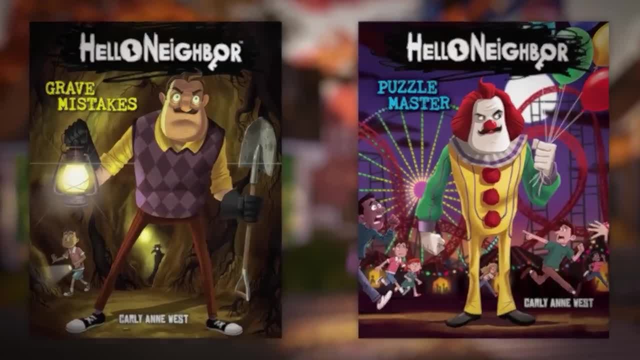 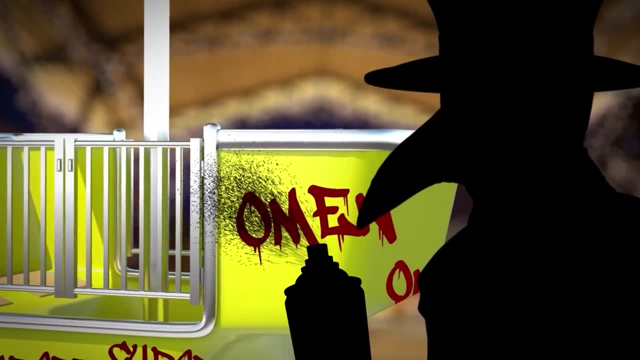 anyway, during the events of both grave mistakes and Trollmaster Mr Peterson, son Aaron and his daughter mya start to investigate the forest protectors. and so the forest protectors begin to sabotage Mr Peterson's amusement park rides. we're feeding them with these words to try and warn him to stay away. of course, 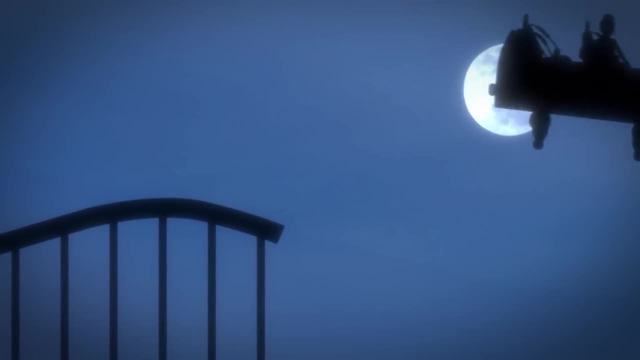 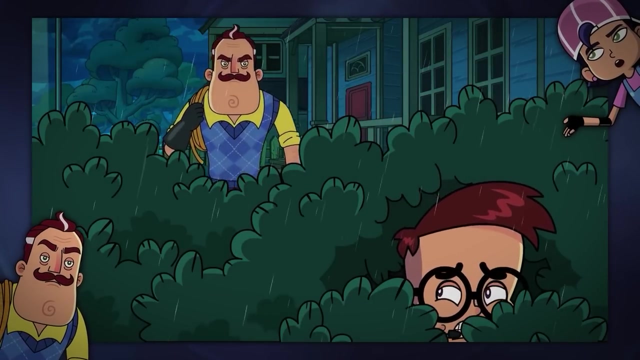 They don't listen, which leads to one of mr Peterson's rides malfunctioning, killing a young girl. This would seem to imply that the forest protectors are at play here, But not so sure. remember, this series seems to be paralleling the books, But it's not one for one. this looks to be Aaron's bedroom. notice the small baseball cap over on the side, so it feels very strange. 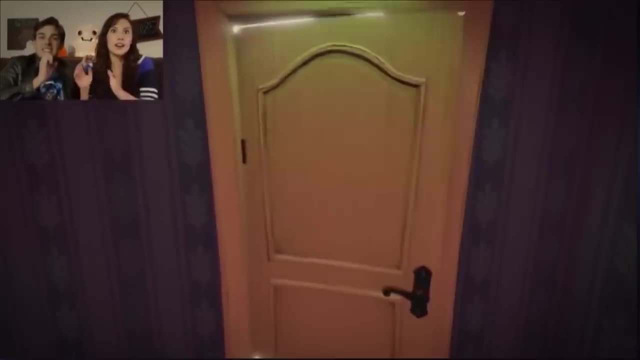 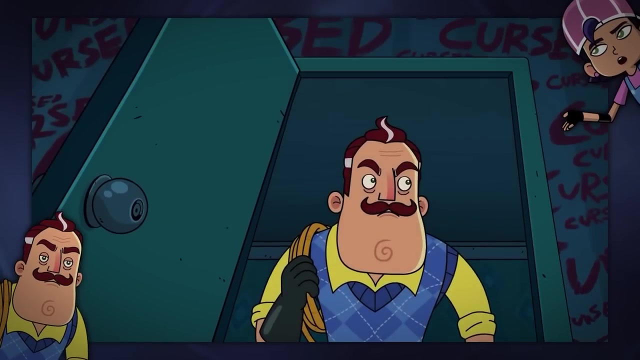 strange for the forest protectors to be inside of the Peterson household, especially given how protective we know the neighbor is. So what then, is this all about? Well, I think all this wall art is down to the neighbor himself. A couple shots later we see Maritza backing up against a wall. 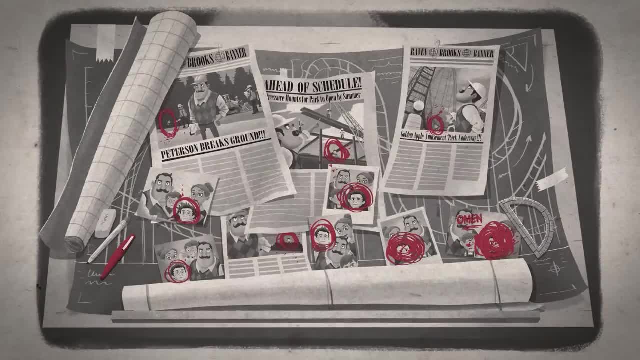 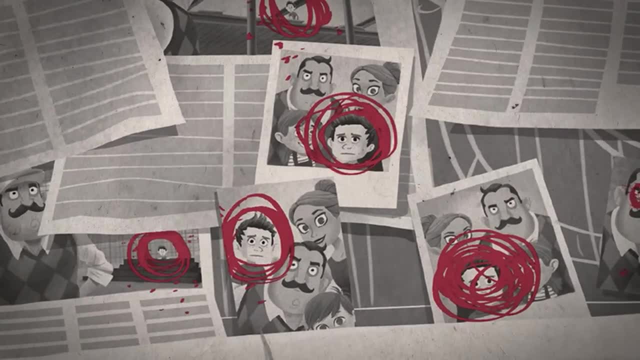 with dozens of newspaper clippings and characters circled in red. This is taken straight from the first book, and it's not just any character that's circled, it's Aaron. Mr Peterson is looking back across everything that went wrong with the park and noticing Aaron at every turn. writing the 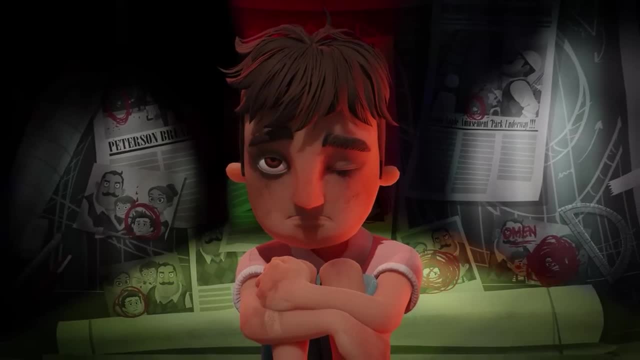 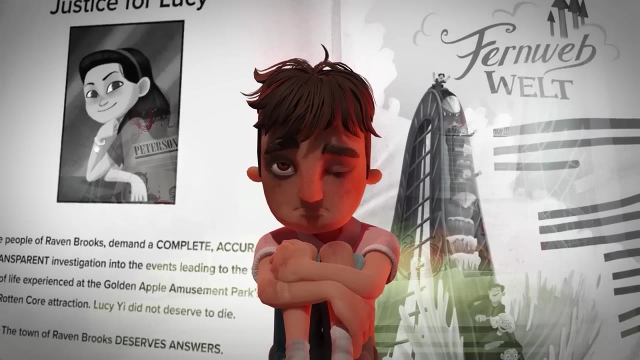 word omen next to him. In his paranoia, he believes Aaron is the bad omen. Aaron was around the ride that failed. Mr Peterson's past rides at other parks also malfunctioned, killing even more people. and surprise, surprise, Aaron was there too. But the final nail in the coffin here, Aaron was also the 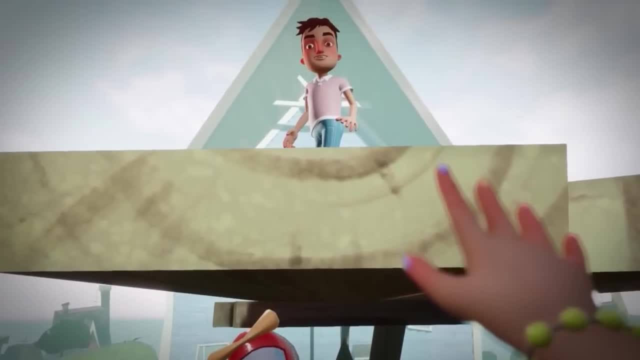 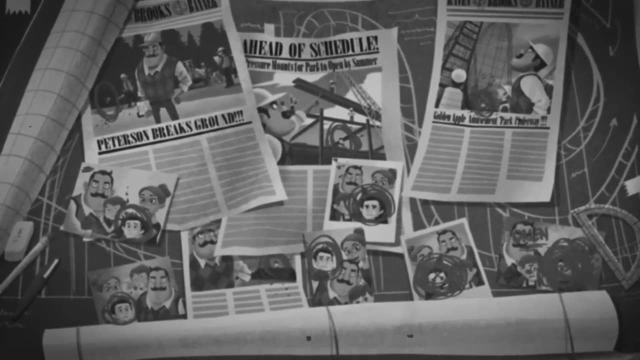 one who pushed Mr Peterson's daughter Maya off the roof, leading to her death. I suspect that that is why he wrote all over Aaron's walls as a reminder of why he was locking Aaron in the basement, meaning Aaron is likely still in the basement of this story as well. But speaking of 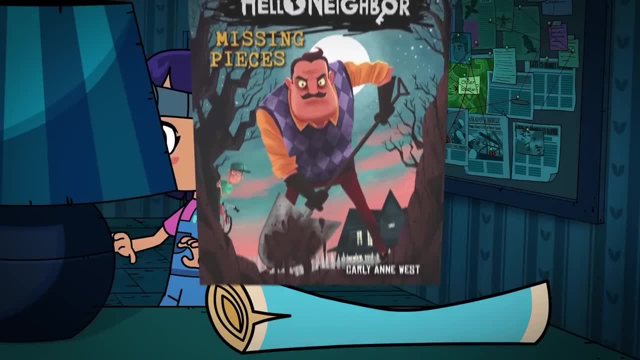 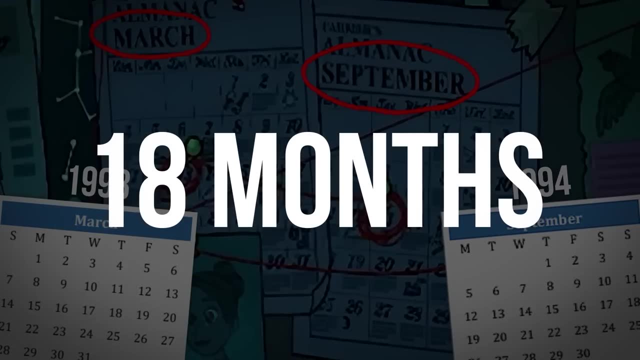 that conspiracy board. while I said it's lifted straight up, I don't think it's a conspiracy board. There are noticeable differences. Some of them are small, like the calendars lining up with March of 1993 and September of 1994, which is 18 months apart. That right, there is the same amount of time. 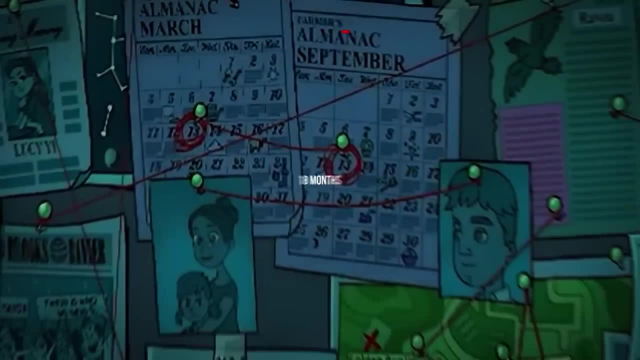 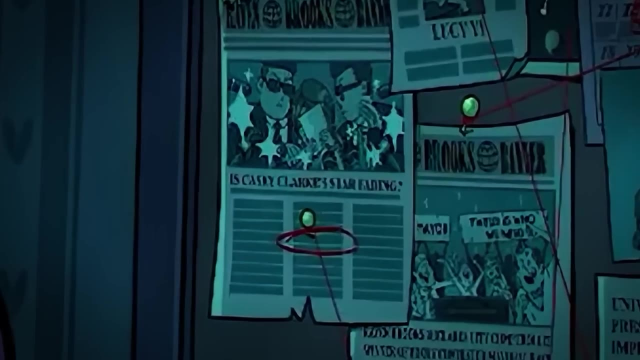 Mr Peterson was given to complete his park attractions in the books, But there are other details here that have themselves a much deeper meaning. We see articles about crows, the university president, committing tax fraud, and a celebrity called Casey Clark who fell from grace. I looked. 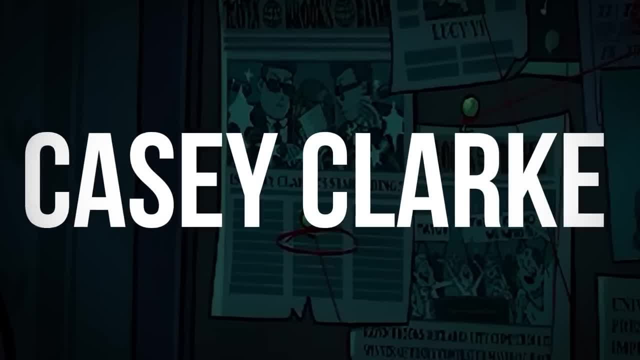 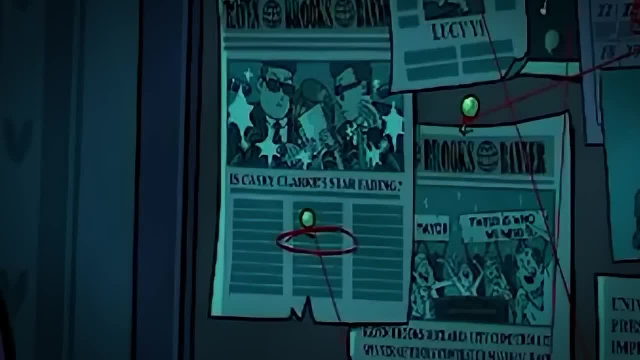 into that character specifically, but she isn't anywhere else in this franchise at all: No books, no games, not even in the animated series, At least from what I could tell- Which means that it's not the character that's important, but rather what they did. 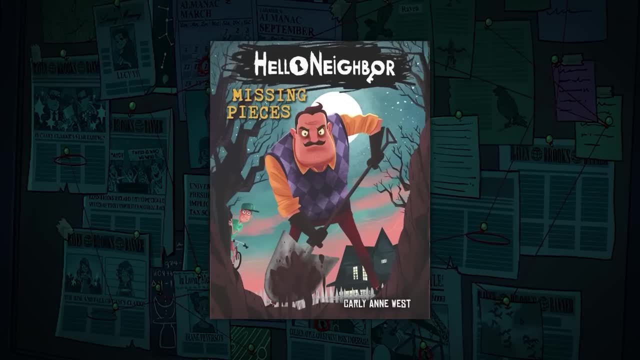 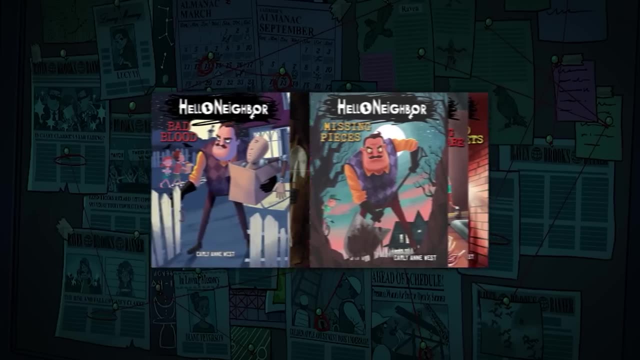 This board isn't just noting down a bunch of paranoid ramblings of Mr Peterson, like we see in the first book. Instead, it seems to be more in line with his investigations during the second book trilogy, which, confusingly enough, takes place before the first book trilogy. 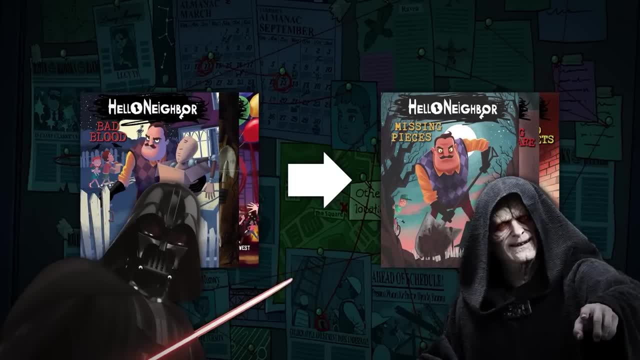 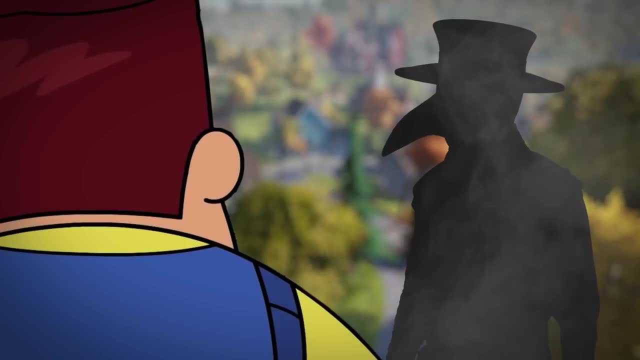 It's kind of like Star Wars if it didn't have cool laser swords and magical powers and instead had a lot of bear traps and boxes- Just so many damn cardboard boxes. It seems to me that Mr Peterson is trying to uncover the mystery surrounding the forest protectors and how they create the 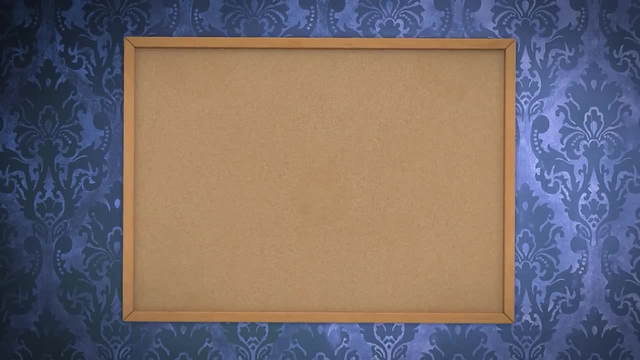 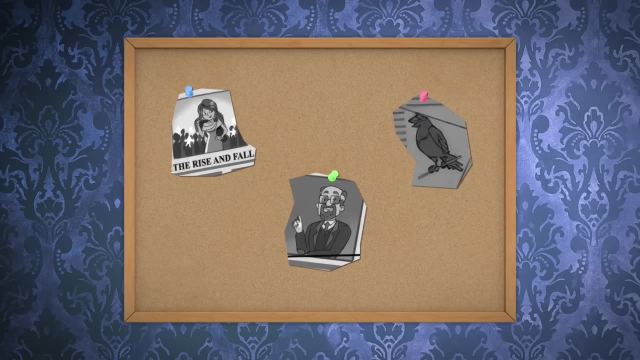 bad luck for the town, while keeping all the good luck for themselves. He's looking into the bad luck that follows people in the town, like the celebrity and the university president, as well as researching into crows, which we've established are a symbol of bad luck. 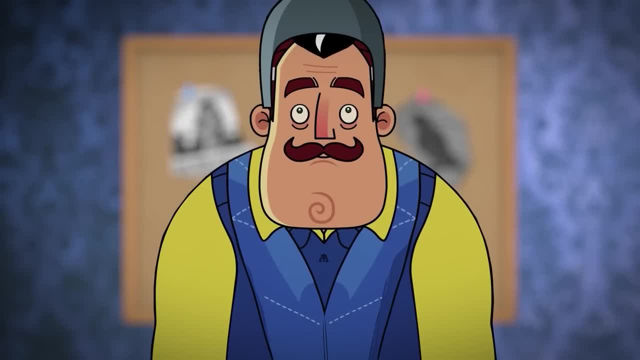 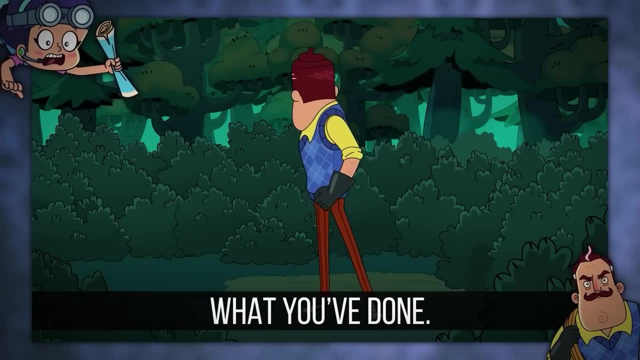 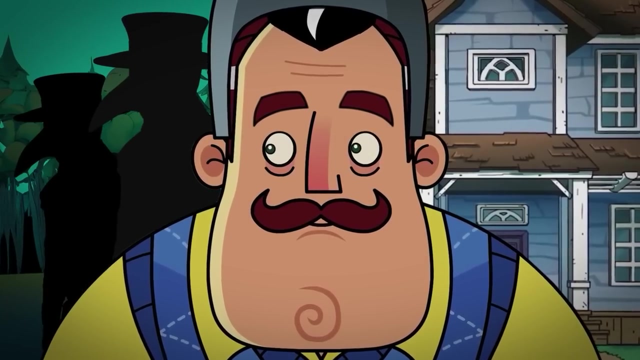 Which makes Mr Peterson a lot less evil and a lot more like a misunderstood sympathetic villain. He literally tells the kids later in the pilot: You kids, you have no idea what you've done. This must be what he's referring to. They're messing with his investigation. I suspect that Mr Peterson feels like he's been cursed by these forest protectors. 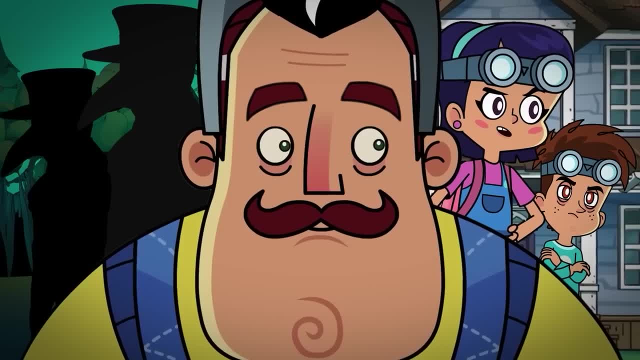 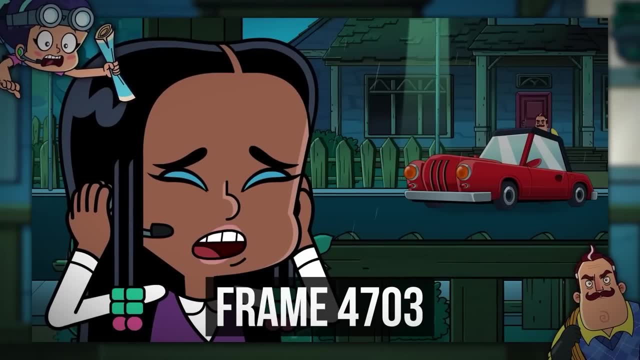 And he's trying to expose them. But he's worried that all these detective kids getting in his way they're gonna not only ruin his life but also ruin the town as a result. Frame 4,703.. That, uh, that walking animation is really something. His body's always turned to the left and we can't see his legs. 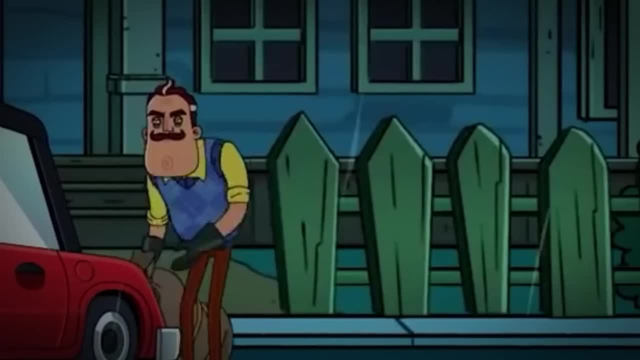 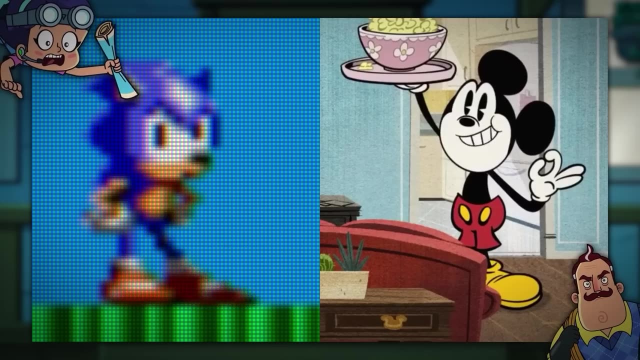 Makes it look like they've used a forward walking animation but just keyframed it sideways, And that's weird because they've shown front-facing versions of him before. So it's not like a Sonic the Hedgehog or Mickey Mouse situation where they always have to face one side or the other because of that iconic shape. 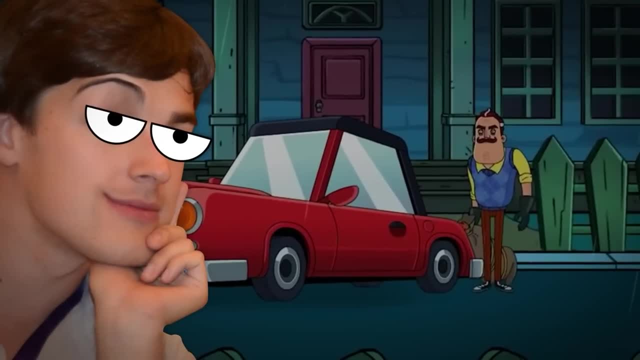 Hopefully they were able to do that. Hopefully they were able to iron that out in the full series. Other than that, yeah, nothing really to add. It just made me laugh. These are the little details that you notice when you're asked to do things frame by frame. 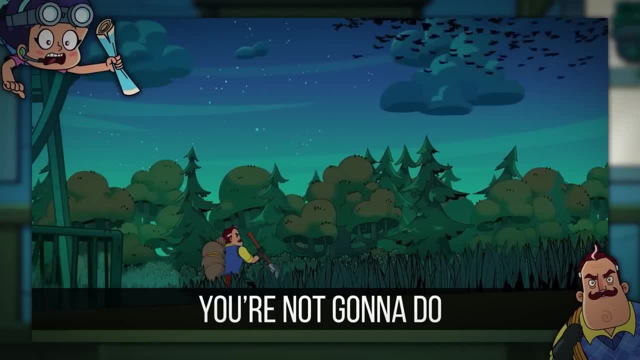 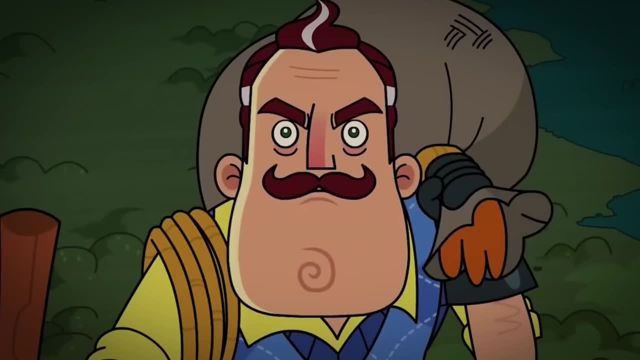 No, not this time, Not this time. You're not gonna do this to me again, Not again. And just like that we're into our final scene And I gotta say the neighbor is far less scary as soon as you make him speak. 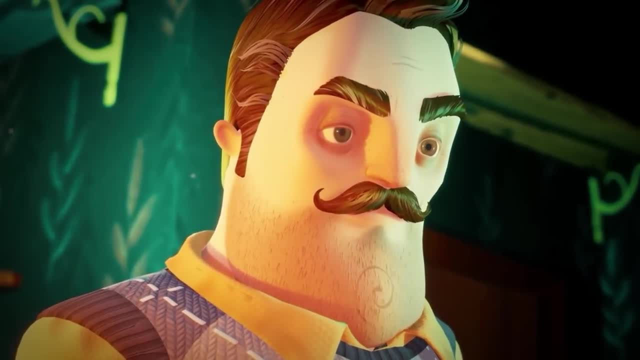 Part of what was terrifying about him in the games, and even in the first trilogy of books for that matter, is that he almost never speaks. In the second and third book especially, he just towers over Nikki without saying a word, Just staring. 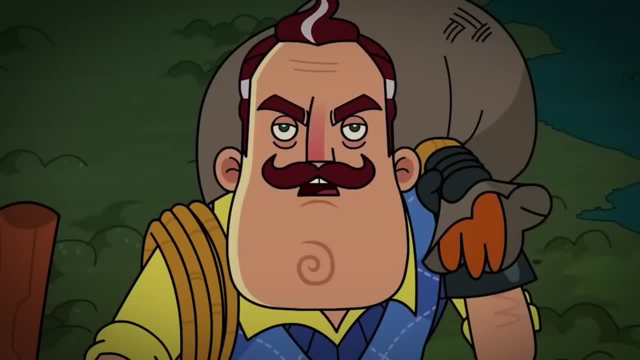 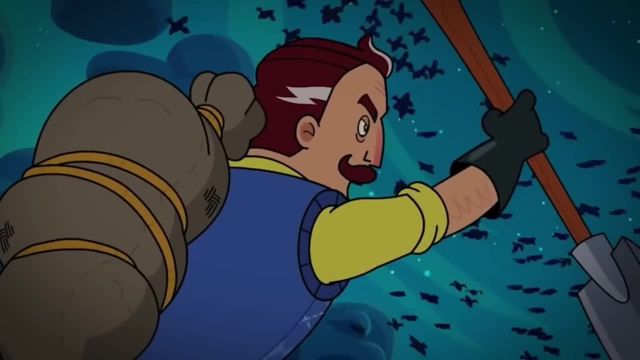 That makes him cry, That makes him look creepy and mysterious. But as soon as he starts talking in full sentences like this kinda ruins the mystique, Makes him a lot less threatening. I get that he's human and they're trying to make him more sympathetic, but I don't know. it just kinda takes the wind out of the sails there. 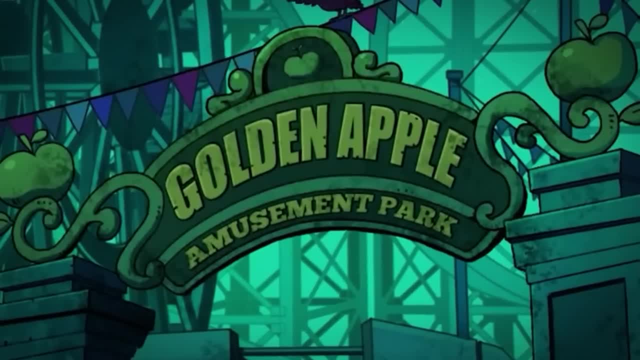 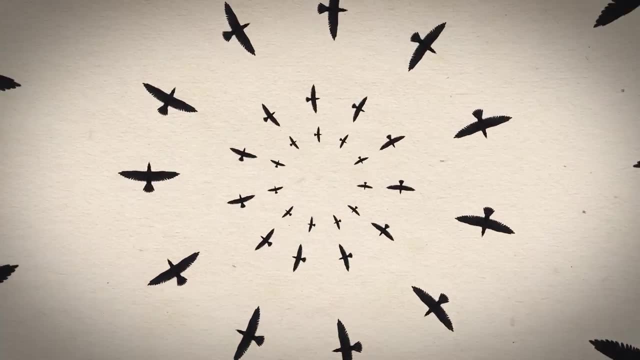 Anyway, we're back at the Golden Apple Amusement Park, which really is the linchpin of the series. So much happens here in the book series and we're clearly seeing some of that take place here. The crows begin to circle, and in the second trilogy of books, crows only begin to circle during storms. 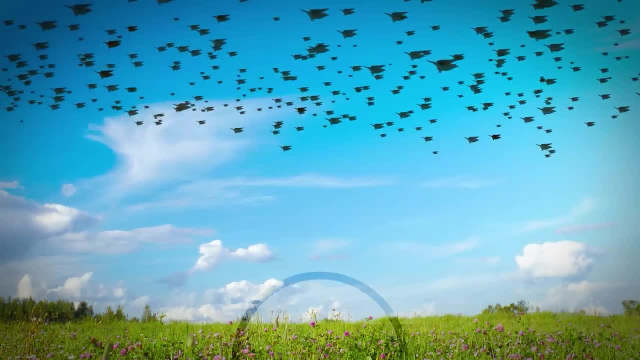 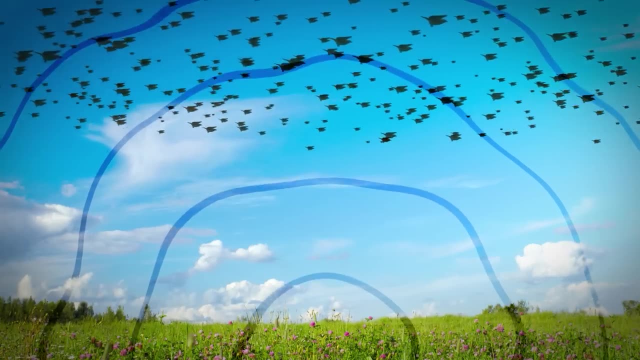 Now, the crows themselves aren't strictly involved in anything nefarious In the books, and in reality, birds actually use the Earth's natural magnetic field To help navigate their way, namely during seasonal migrations. Messing with that field, though, can cause an effect known as electro-smog, which causes birds to break away from their traditional flight paths. 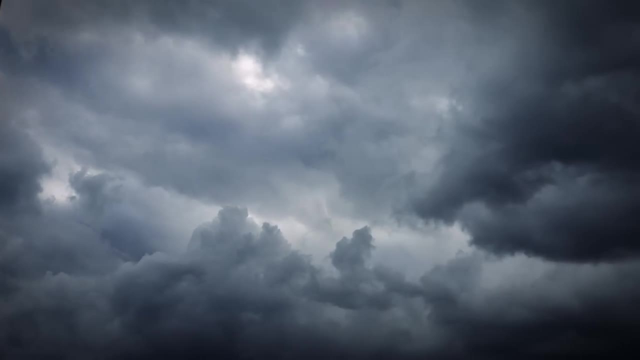 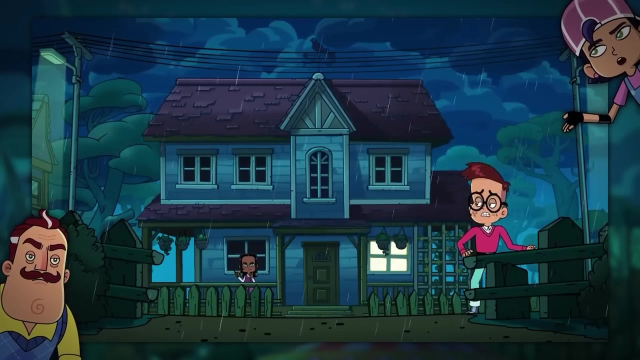 Now, really big storms do have the ability to affect electromagnetic fields in the world, but never really enough to affect bird migrations. Here in Ravensbruck, though, they're known for having incredibly powerful storm systems compared to the rest of the country. 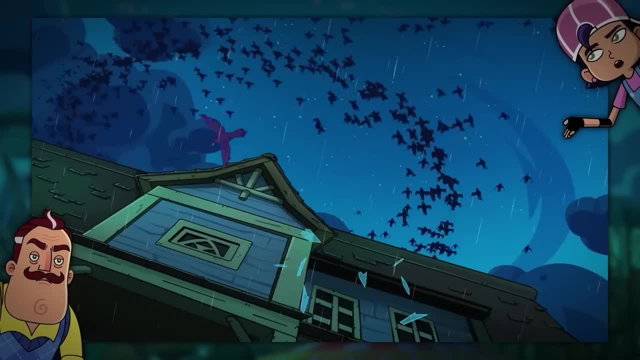 Which, in turn, causes the crows' flight patterns to shift drastically, leading them to then circle. However, this also acts as a sign of a storm coming, and when a storm comes, that means the force of the storm is on the way. 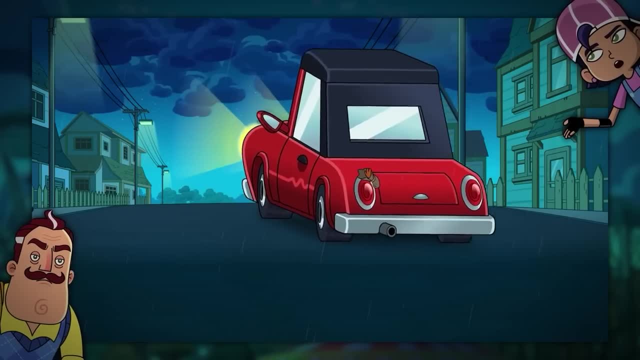 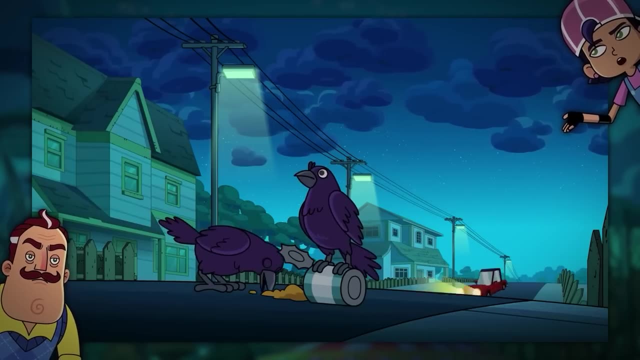 That means the forest protectors have begun their ritual to curse the town and thereby bring themselves good luck. That's why we see Mr Peterson here yelling at the sky: You're not gonna do this to me again. It's not the crows that he's speaking to, but rather the forest protectors who are bringing a curse upon him and the rest of the townspeople. 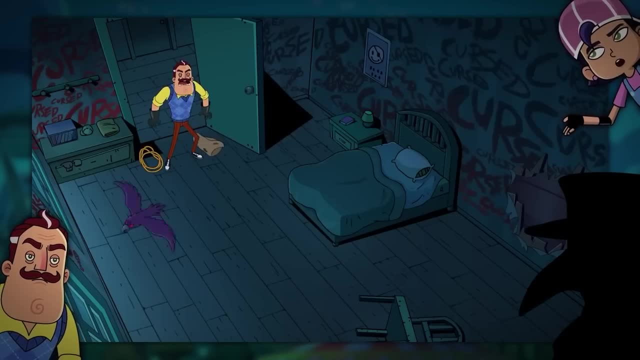 Which he blames for the death of his wife, his daughter Maya, and the failure of his ride designs. Later in the scene, we see him reveal an object with a gemstone in the middle, which is another direct reference to the forest protectors and their ritual. 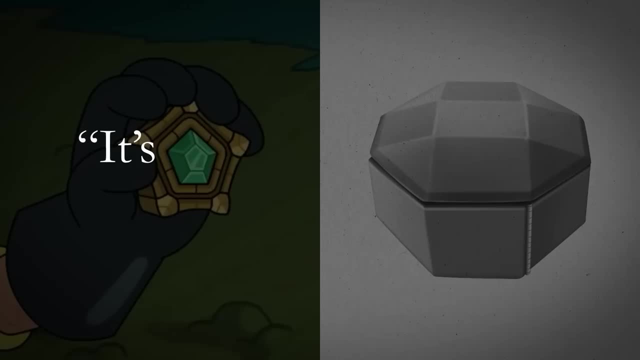 It does look slightly different in the books, but clearly it's meant to be the same thing. Quote From here: it looks to be about the size of my palm, a tarnished, brassy thing, And just look at the pictures. clearly there are some obvious comparisons here. 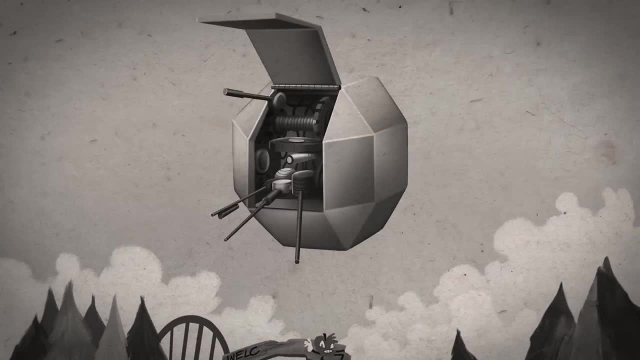 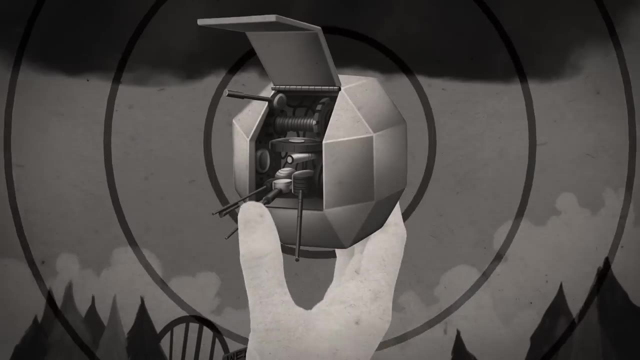 Now, this device in the book is super important because it's part weather detector. This allows the forest protectors to know when a storm is coming so they can perform their good luck ritual, But it also seems to be the thing that actually brings good luck to anyone who's holding it. 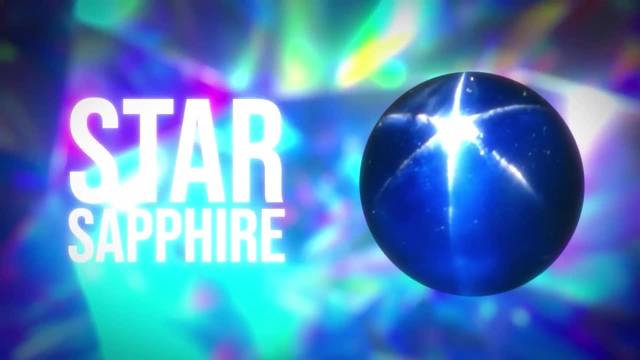 I wonder if that's maybe why it changed its shape. There are these real world gemstones called star sapphires. They look like normal sapphires but with a star-shaped pattern in the middle. Back in the day they were thought to ward off witchcraft, hexes and curses. 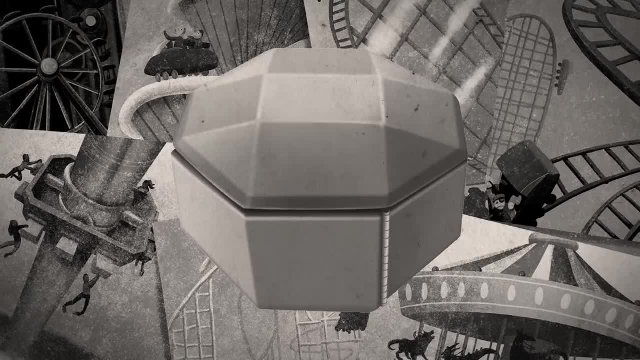 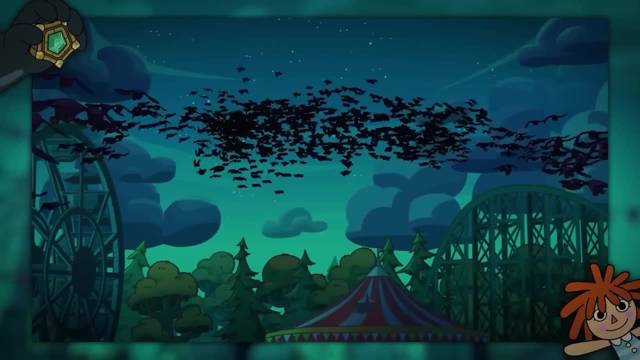 Now in the book, Mr Peterson managed to make one of these and suddenly the investigation into his past ride malfunctions and all the deaths that they caused- they all get dropped in an instant. So again, this seems to be what he's referring to here when he talks about the forest protectors not doing this to me again. Because he now has the device that'll be able to change his fate. But one thing you'll notice throughout my analysis here is the repeated phrase in the books. in the books, right, All of this stuff is explained in the books. So I just wanted to see if there was anything I could take away. 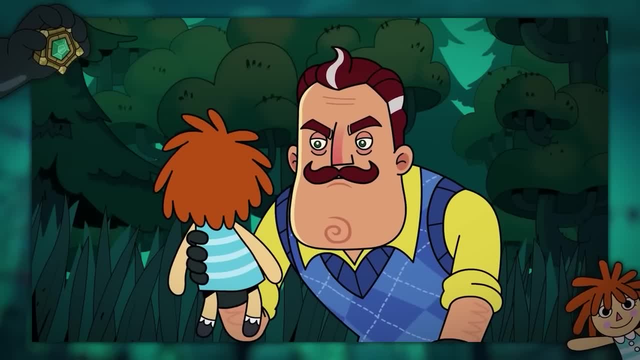 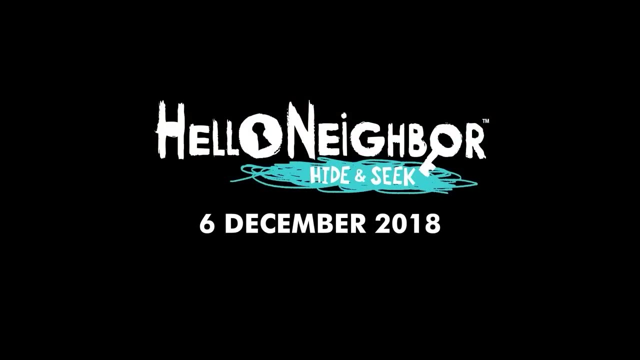 From this scene that didn't rely on book knowledge, And the thing that stood out to me was the burying of the doll in the middle of the amusement park. This doll was Maya's doll that we see her carrying around in the game Hide and Seek, which came out in 2018.. 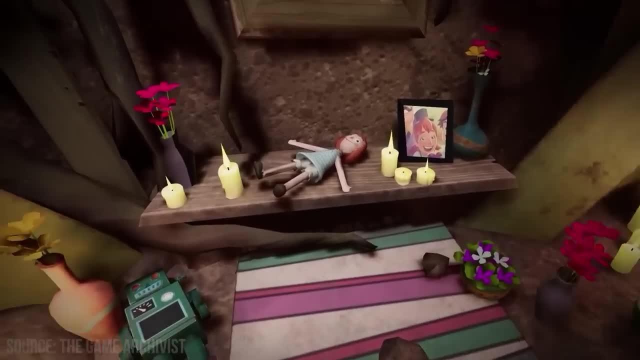 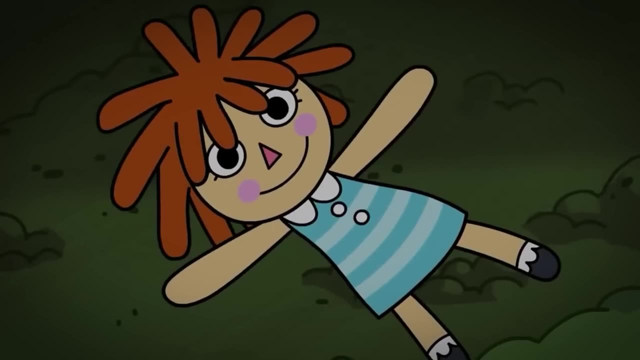 Now this doll has shown up in later games of the franchise, like in an underground shrine during the VR game Search and Rescue, But Mr Peterson's never buried this doll specifically in any of the other games or stories, as far as I can tell. 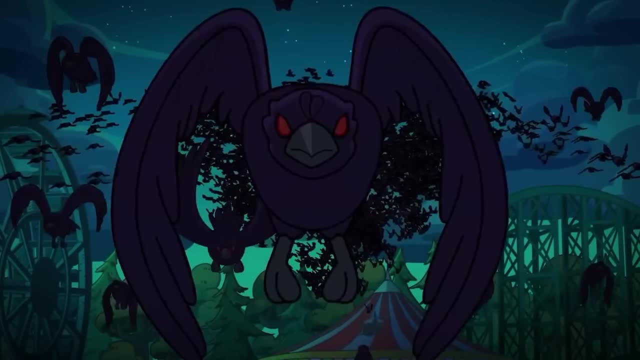 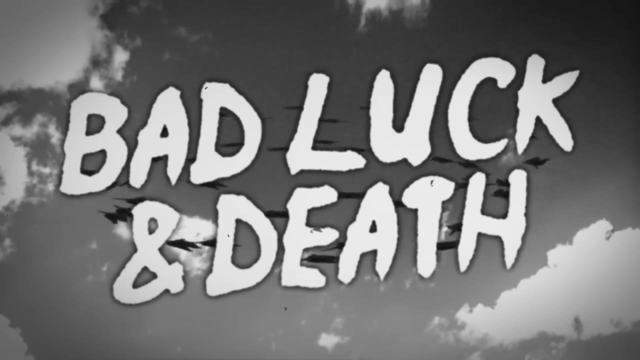 So why change that? Well, I would imagine that they're expanding on the Crow lore, Which kind of sounds like a joke. but I'm being completely serious here. I mentioned at the start of this episode how crows were a sign of bad luck and death. 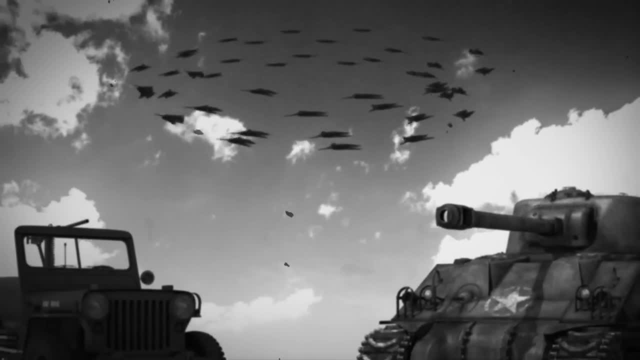 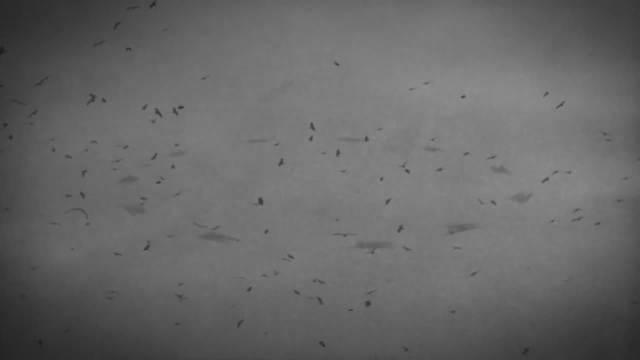 Part of the reason for this was because crows would circle battlefields after a war, looking to feast upon the dead that lay across the land. However, there is another potential meaning if you see crows circling, A more spiritual meaning. One interpretation of crows circling, like we see, is that there's a spiritual transition between our world and the spirit world taking place. 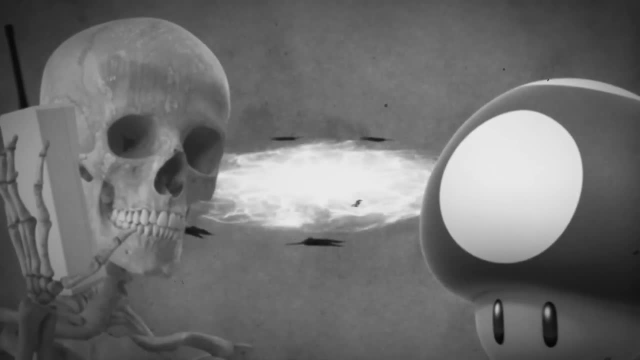 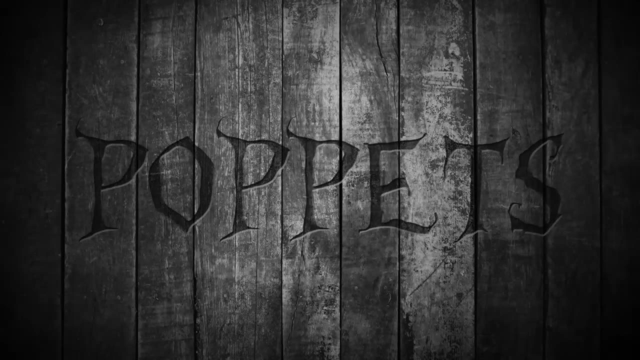 This can be as simple as someone communicating from beyond the grave, but it can also be a symbol of rebirth And you see, this is where the doll comes into play. These dolls have a spiritual element to them And we see that in real world with puppets. 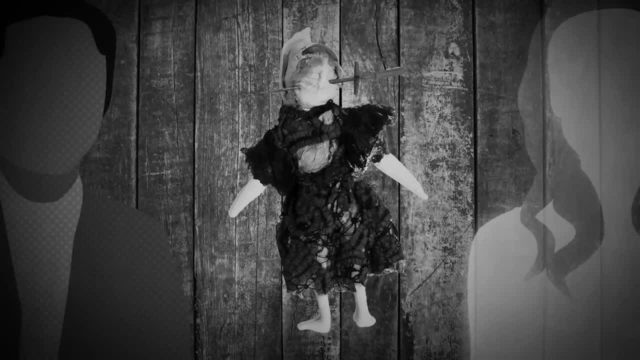 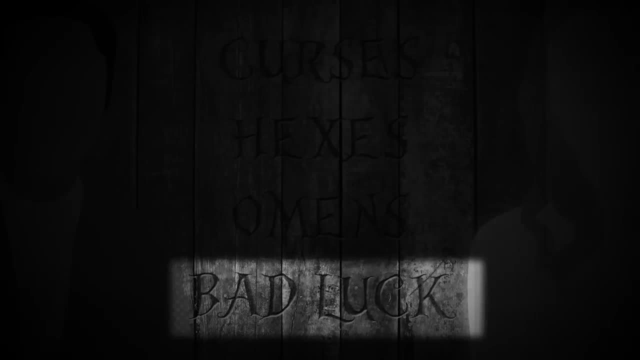 Now, puppets are meant to serve as a bridge between humans and the spirit realm, Allowing the user to remove the effects of curses, hexes, omens and even bad luck. And hey, would you look at that? There's that whole luck thing again. 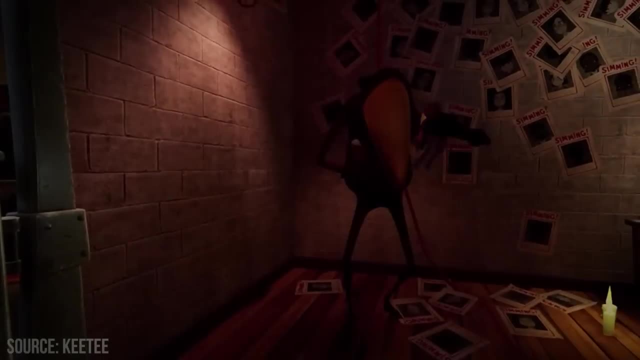 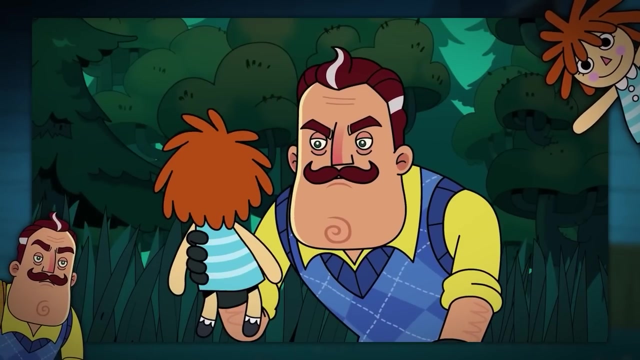 The VR game Search and Rescue actually uses dolls in a similar way. In the final level of the game, Aaron is able to use a doll of another character to switch between his own body and theirs. The dolls have a spiritual connection to them, And when you combine that with the crows circling- 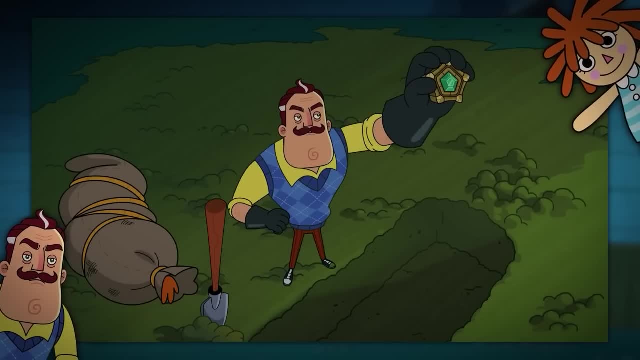 we see that Mr Peterson burying Maya's doll and using the good luck device from the book is all part of some kind of ritual of his own, Either trying to bring him and his family good luck, like we see in the books, or maybe it's something darker than that. 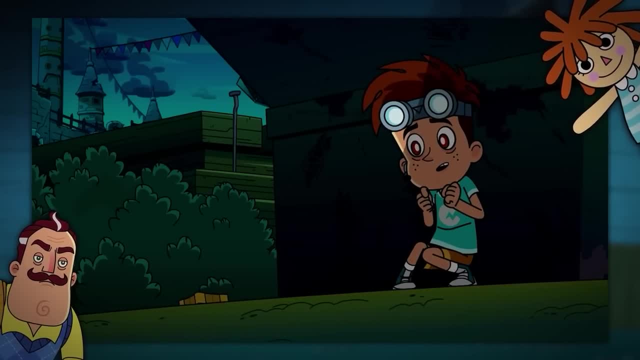 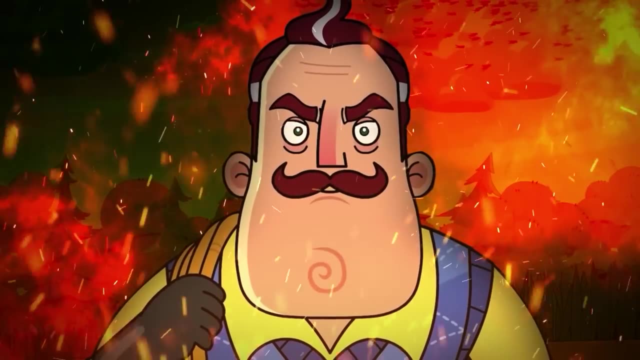 Maybe he's trying to reach out to the spirit realm and bring his daughter back to life. We saw in the original alpha that he is more than happy to make a deal with the devil. Who's to say that he wouldn't try something so extreme? that stands against both God and nature. 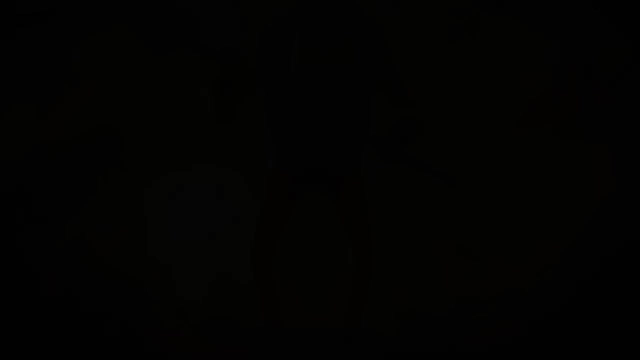 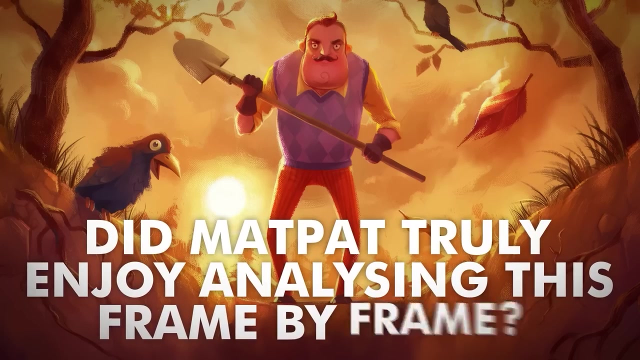 And that, my friends, basically brings us to the end of this pilot episode. So it's time for me to finally answer the question that I've been wondering for the last four years: Did MatPat truly enjoy analyzing this frame by frame? And I gotta say, yeah, it was okay. 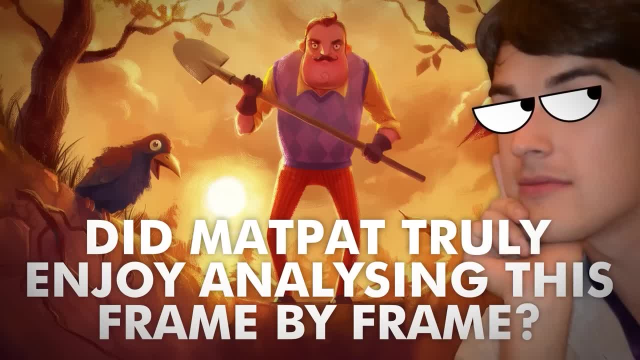 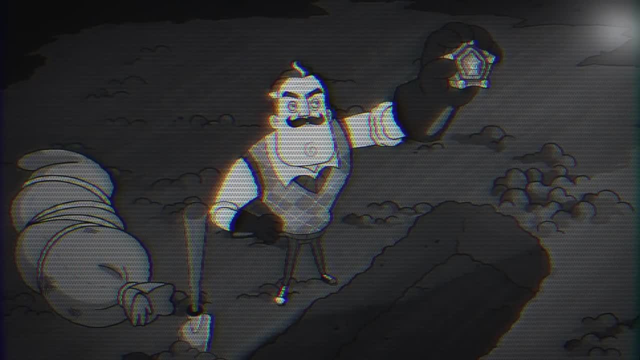 But honestly, I would have enjoyed it way more if the lore of the books was actually in the pilot itself. I mean, really think about how this episode's gone If we go back through this video and remove any and all references to the books and the book lore. 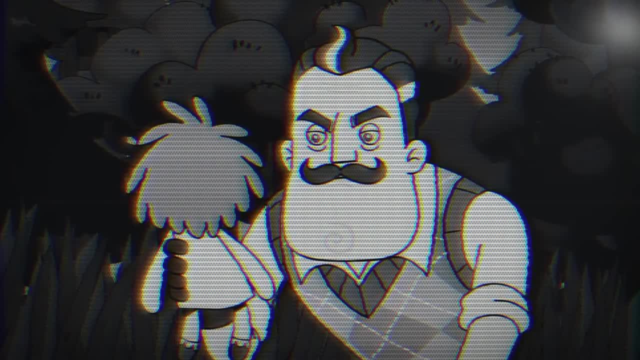 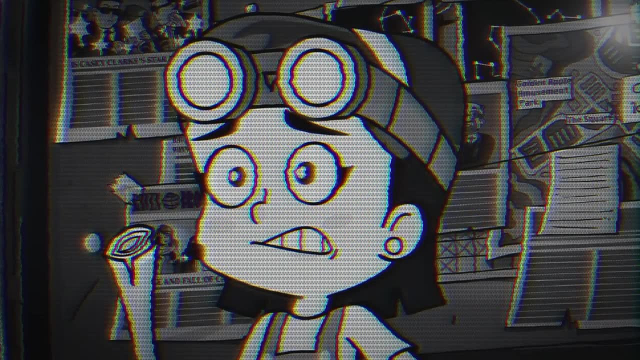 even the ones that came out before this pilot. what would I have actually been able to predict? I guess I would have found some cool details about crows Maya's doll. Maybe I'd been able to figure out some connection to bad luck. maybe. 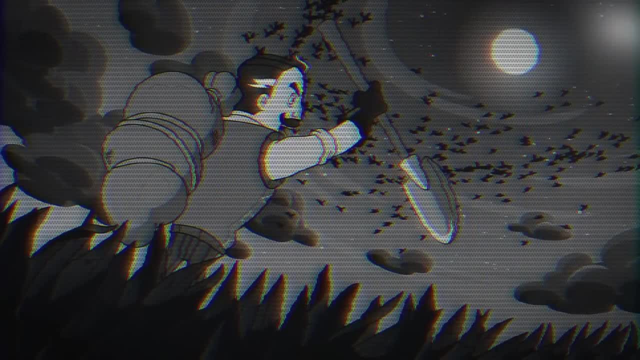 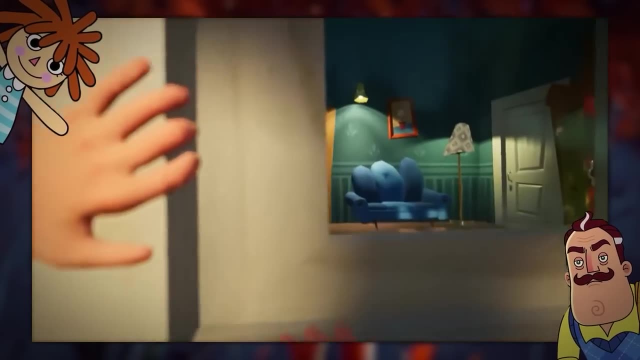 But the idea of a weather detecting good luck, The entire concept of the forest protectors- Yeah, there is no chance. That never appears in any sort of game media. The old days of Hello Neighbor were fun because all the answers were in the actual game itself. 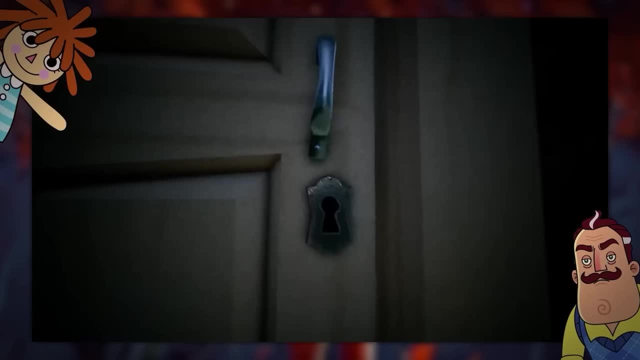 Anyone could just pick up the game and understand it, And for those who were truly dedicated fans that wanted to go a level deeper, all the clues were in the game, minus a few small details that might have been left on a Twitter page or some website. 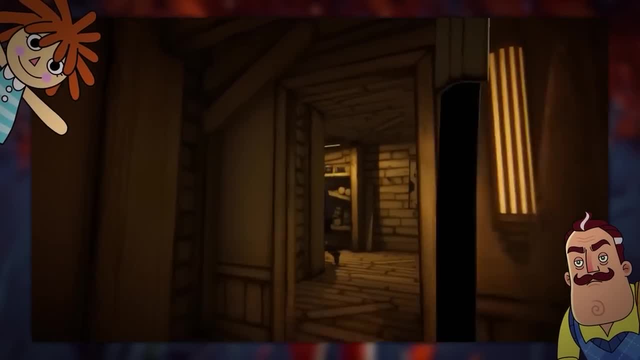 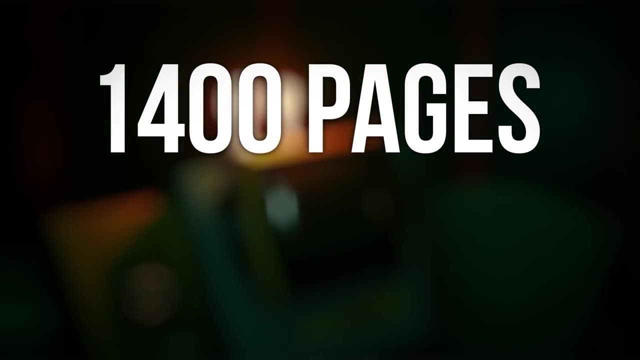 But nowadays, all these indie horror franchises, they're basically asking us to do homework, Because to understand anything in this pilot or, honestly, the recent games, you have to have read the 1,400 pages spread across their seven books. Now, to be fair, this isn't just Hello Neighbor's problem. 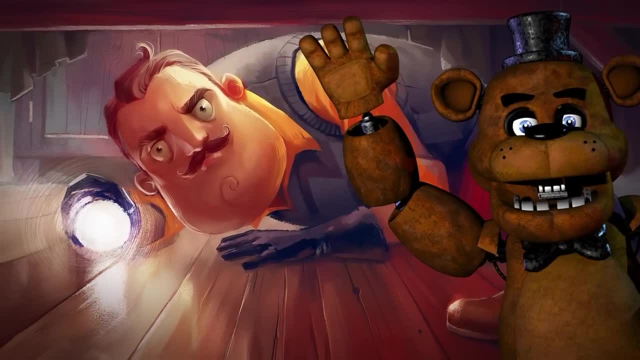 We've been seeing it more and more across all sorts of media- FNAF great example of that. It used to be that the games were completely solvable just from the games alone. Sure, you might be able to find some extra cool information on Scott's website. 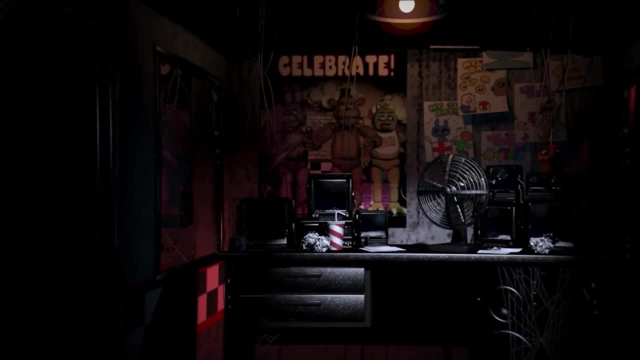 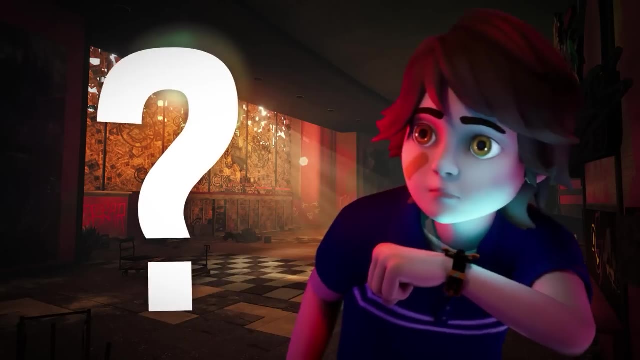 or a cryptic line from a single book, but the game was all you really needed, and it then left you with some dangling threads to theorize about in future games, But, by ruin, Still have no idea who Gregory really is, why he's there. 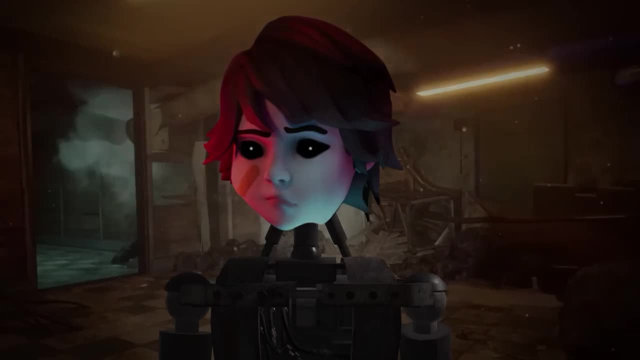 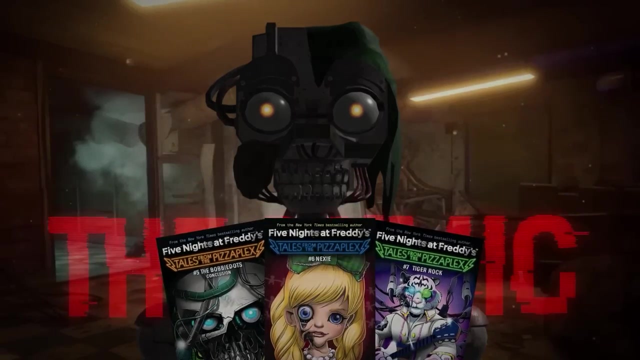 Oh, and now there's this random robot down in the basement pretending to be him. If you only play the games, there's no way that you would know that this thing is The Mimic, the big villain from three of the books, or that Gregory was patient 46 and definitely evil. 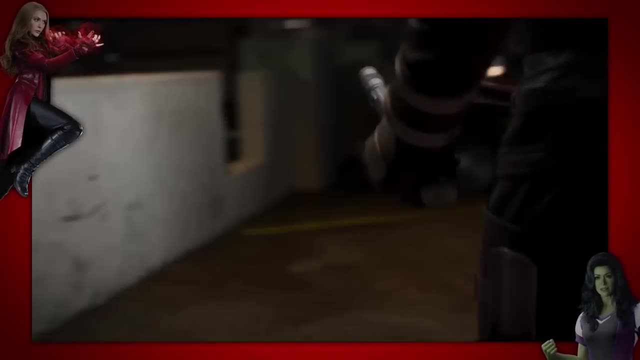 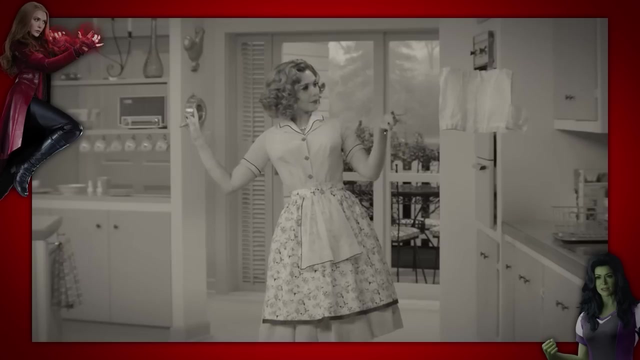 We're also seeing it with franchises like Marvel, who are now so focused on overarching narratives that the individual stories are becoming less contained. And if you do hope to understand everything about the main antagonist, sorry, you gotta binge eight hours worth of television shows multiple times over. 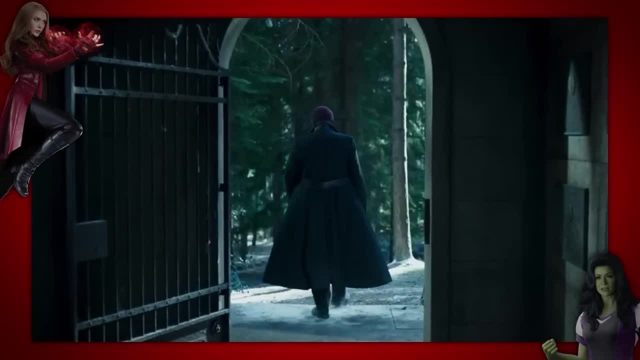 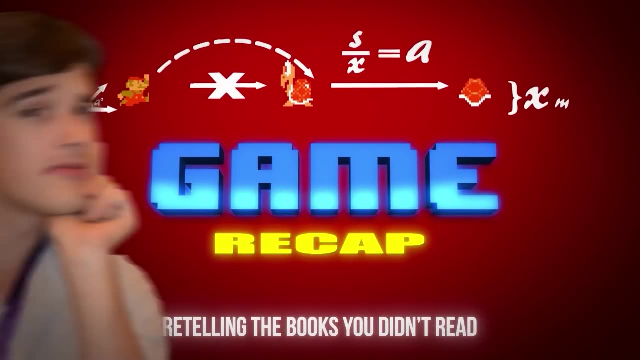 This naturally leads to more frustration and more burden and burnout in the fanbase. Now any theory that gets made stops being a theory and becomes more of a recap of the last few books that nobody bothered to read, which just isn't interesting for me as a theorist. 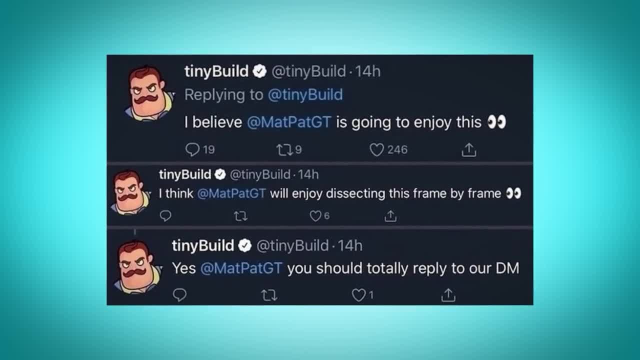 or for people watching these videos. When these tweets initially came out, part of the reason I didn't respond was for exactly this reason. I had my hands full with the FNAF books and didn't have time to catch up on all the extra outside media. 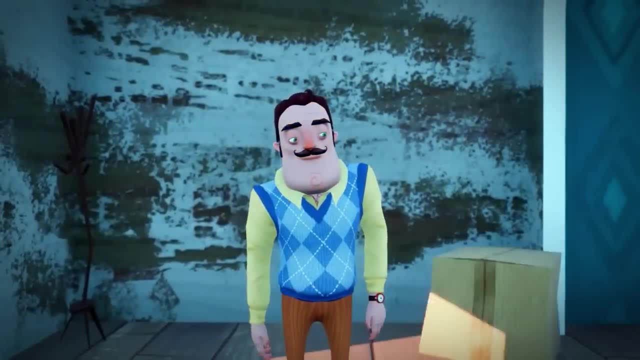 that was being made for this particular franchise. But look, I don't want this to be a complete downer of an ending, because, besides the box stacking and glitchy gameplay, I think this franchise is fun. It's goofy, it's dumb, but it's fun. 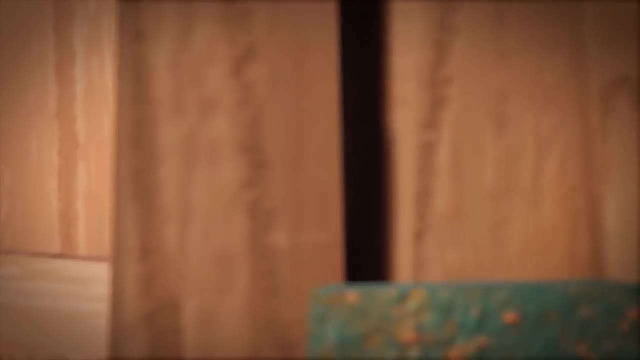 The story in the books is actually a good story. We just need it within the actual games and show, because there's a lot of potential for the future of this franchise. in the theorizing department, From what I can tell, there are more Hello Neighbor games on the horizon.